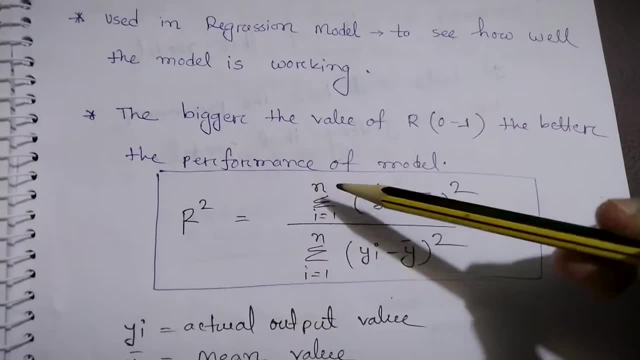 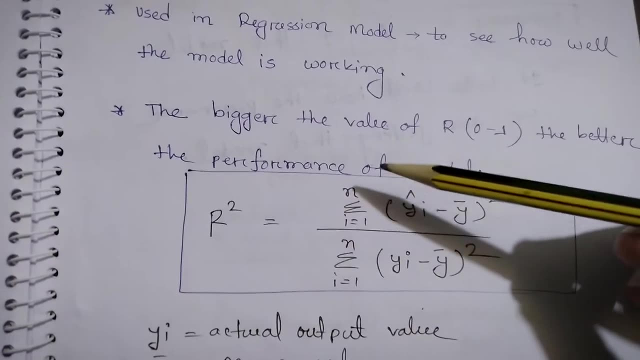 would be. so the formula to find it is: r square is equals to of summation of the value of r squared i is equals to 1 up to n. if this n is the number of given data set, you have. your data set can be 1 000 row, 2 000 row, or 1 lakh row, 1 million row, this type of things. it can go up to n number of. 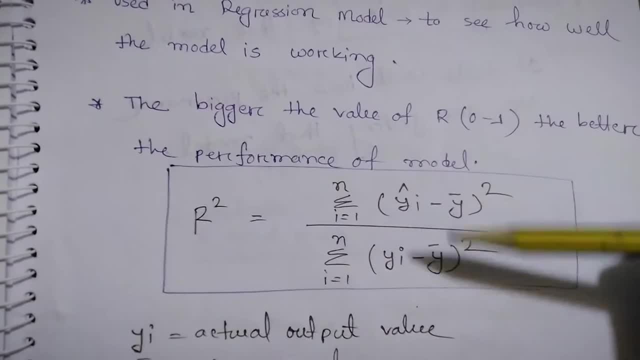 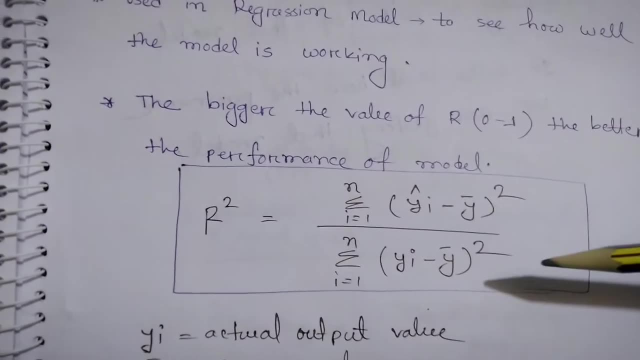 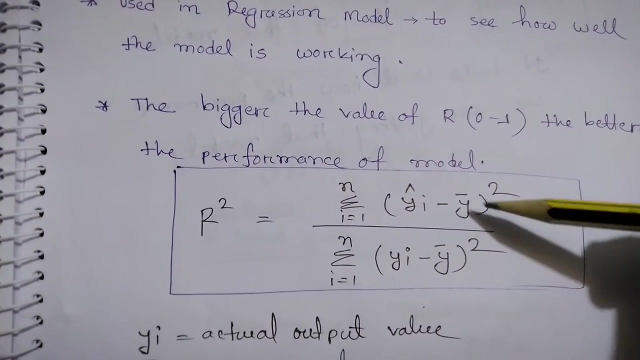 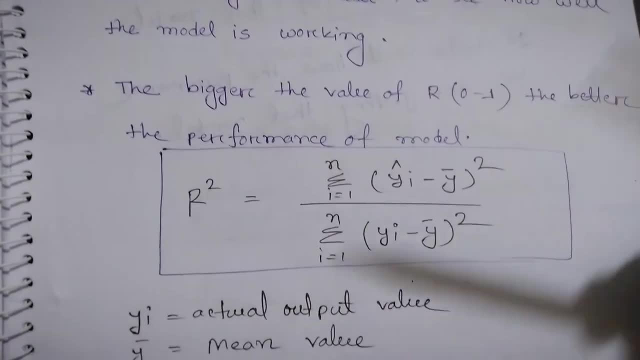 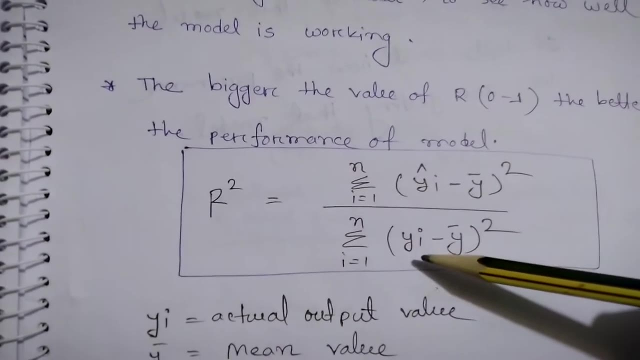 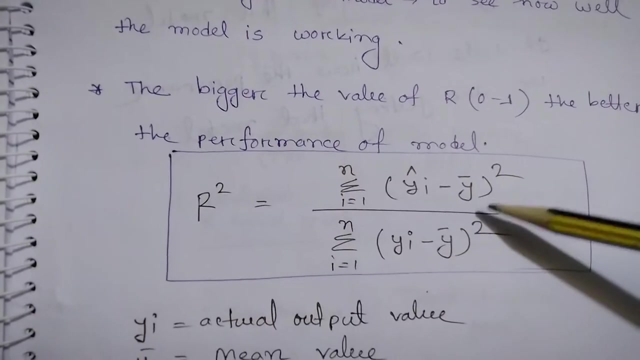 of y, okay, and there is squared. divided by this, summation of i is equals to 1 up to n and y i. this is actually our actual data given in our training data set, not the predicted one. actual data minus the same, the average and their differences and their square. so we are finding the ratio of the. 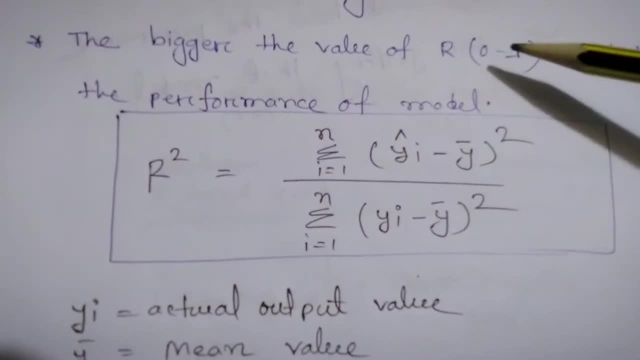 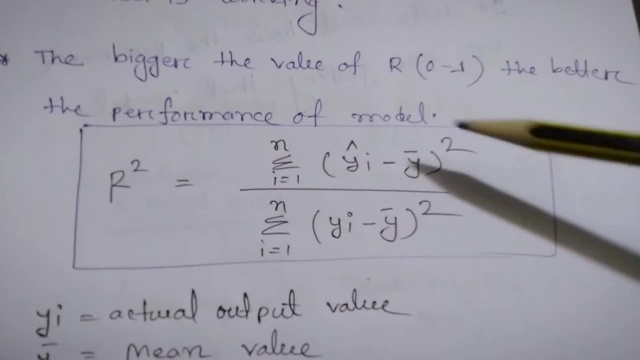 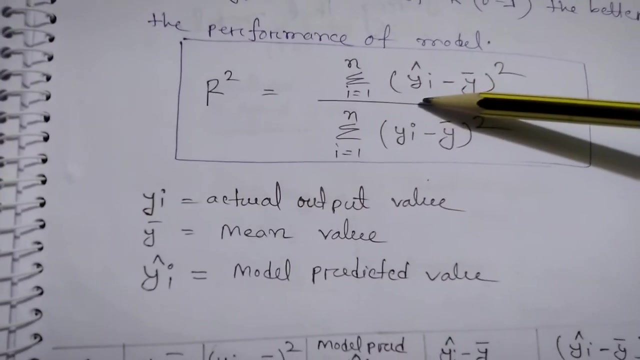 difference of the predicted value minus the mean value, square divided by summation of actual value minus the mean value, the differences and the square. so here, given y, i is the actual output value, this y is the actual y output value. y bar is the mean value of our given data set, or y i cap. 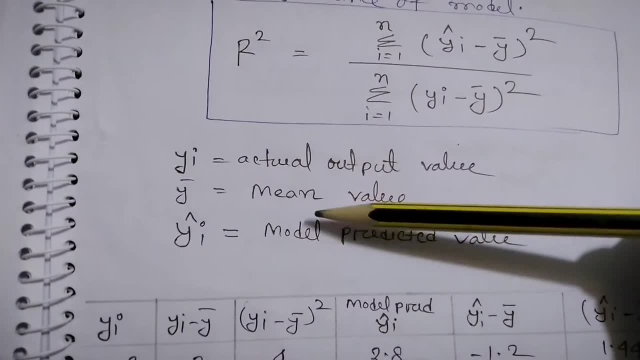 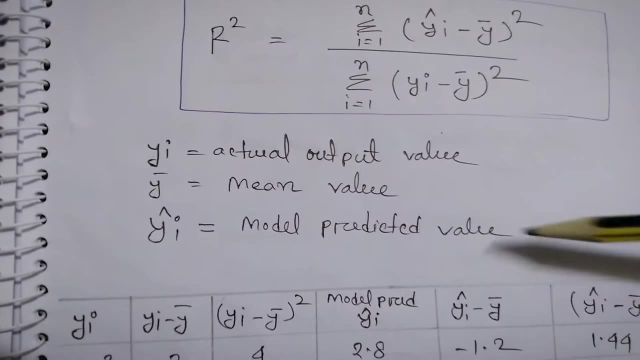 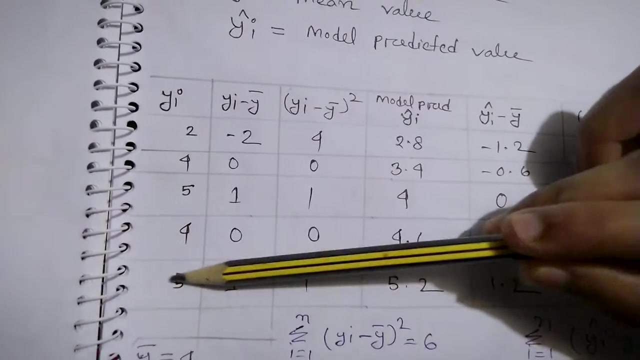 this is the cap sign. it means that it is actually use model predicted value that your machine give based on your training data set. this is actually the predicted value. now see the mathematics of this here. suppose our actual data set y i is 2, 4, 5, 4, 5 and you need to find the difference between y. 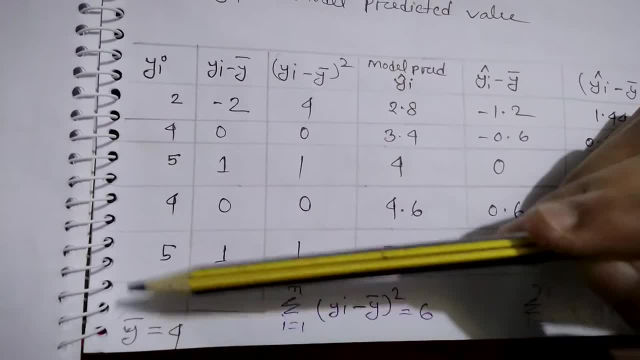 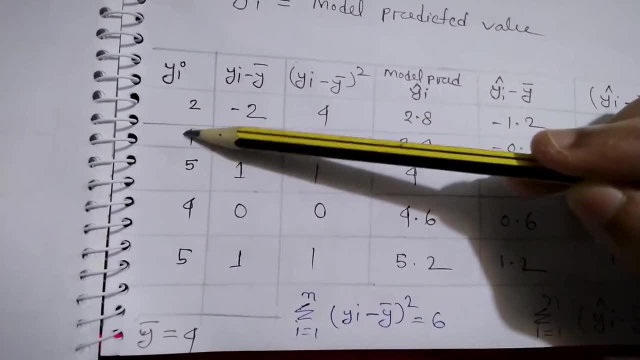 actual data set and subtract it with the y bar. y pi is the summation of all of the data divided by number of items. suppose these all. just add all of those and divide by number of items. one items, two, three, four, five, five items, you get. y bar is equals to four. this is pretty simple and you get: 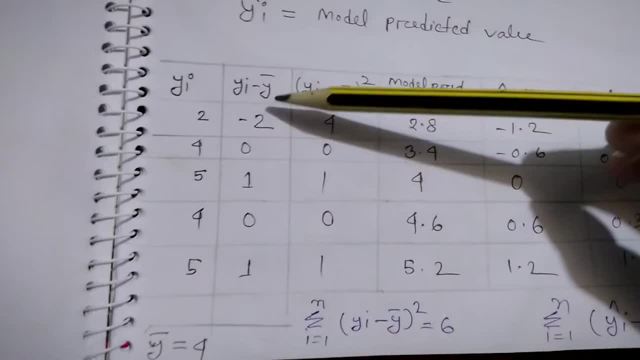 the difference. this value is two minus this value is four. so, minus two, this value is four minus this value, which is 2. 2.mar 0.4. 12.黏: 4 minus this value, which is 0. so in this way you calculate all of those and you need to find the. 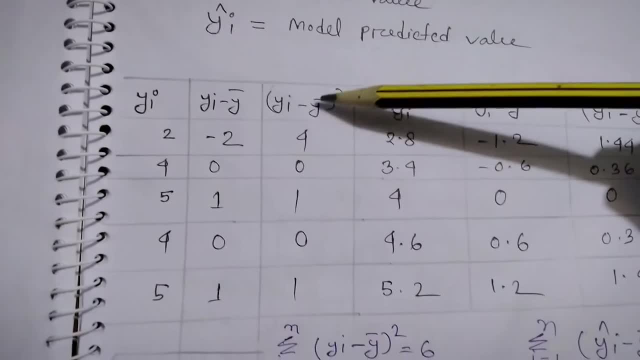 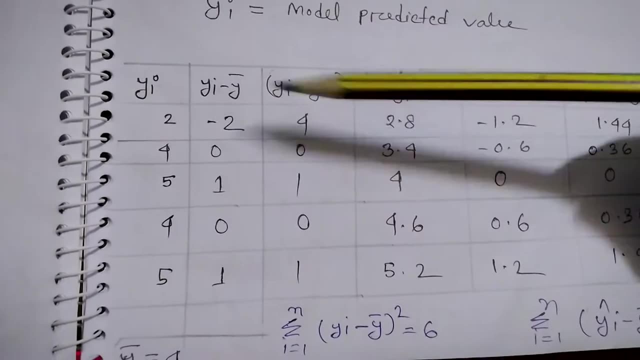 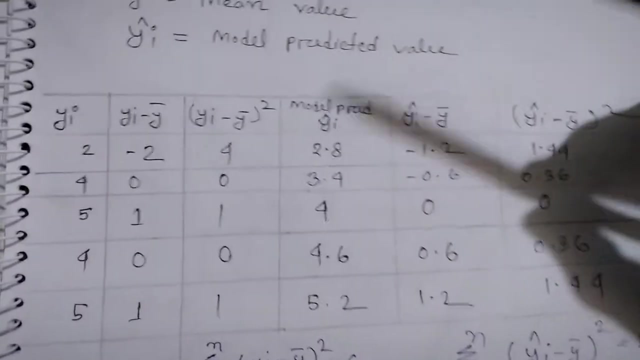 square, so that we do not get any negative value. this is also based on the formula. we need to find the square of them, y i minus y, bar whole square, and this 2 square is equals to 4: 0 square, 1: 1 square, which is also 1. so you just find it very simply and easily, and then you have the model. 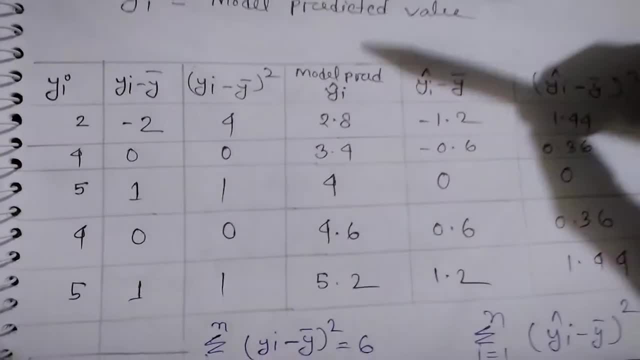 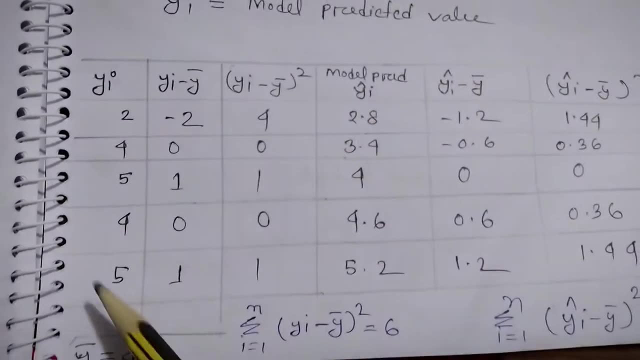 predicted value that your machine learning algorithm give, which is y, i cap it is 2.8, 3.4, 4, 4.6 and 5.2. your actual value is this one, 5, but your model predicted is 5.2, so there is little bit. 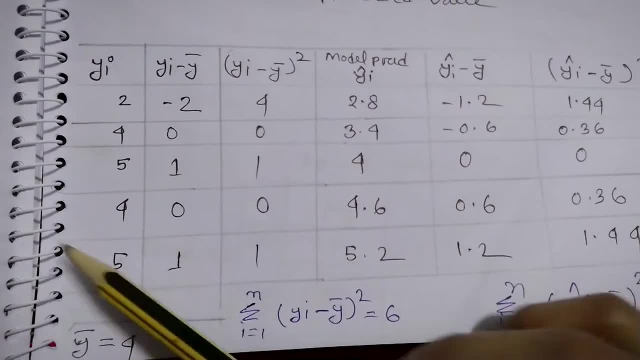 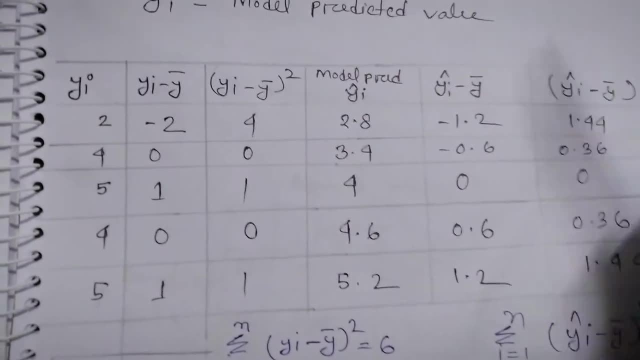 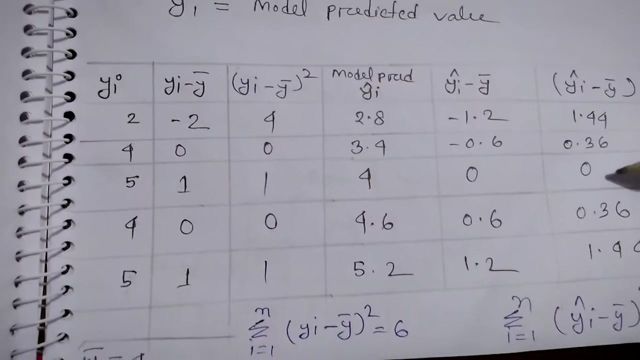 of differences between those two, actual and predicted value. you just need to find the difference and see how much it is perfect compared to this value and this value. we just need to find the more perfect value, compare it and get the most perfect value. this is actually what model predicted value. okay, so we. 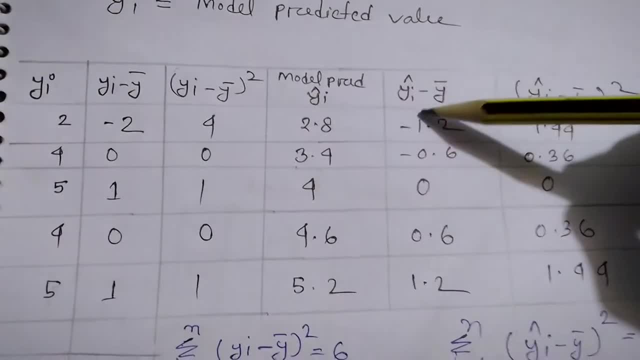 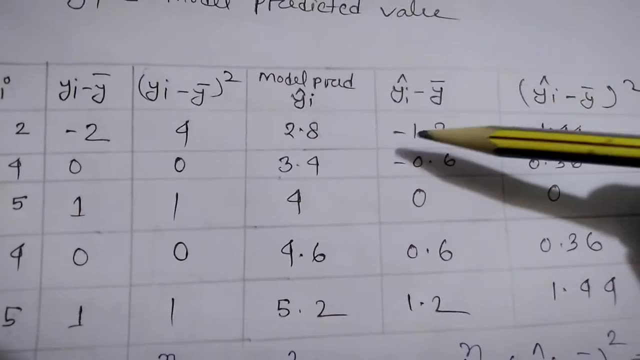 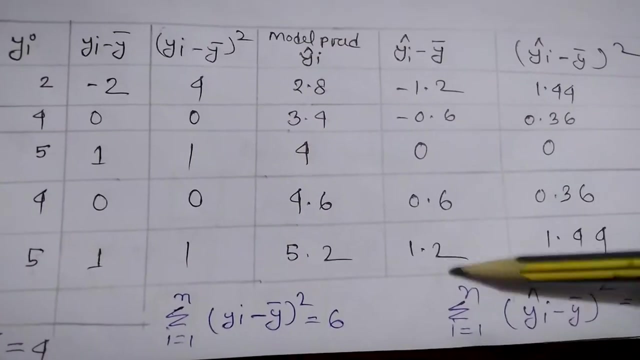 need to find the differences of your model predicted value with your y bar, which is the average or mean. so 2.8 minus 4 is actually minus 1.2. same way, you need to just subtract from this value to this value, this value to this value, and add those things. you just need to find the square. 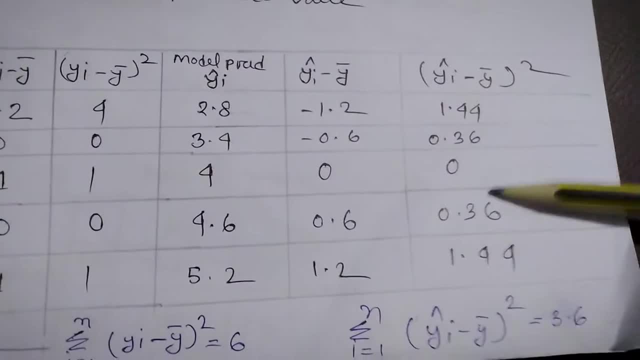 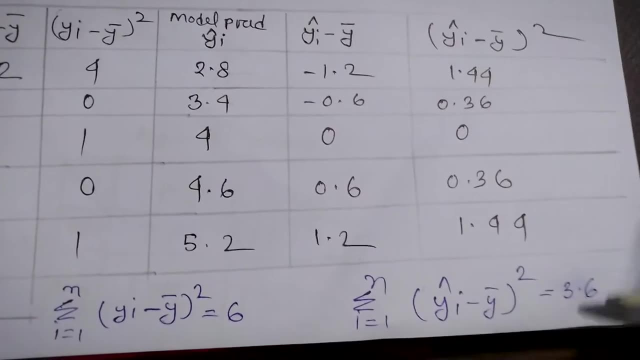 same as this one. just square it and you get all the value and summation of i is equals to 1 to n y. i cap minus y by whole square is 3.6 and in this case summation of i is 1 to 10. summation of i is: 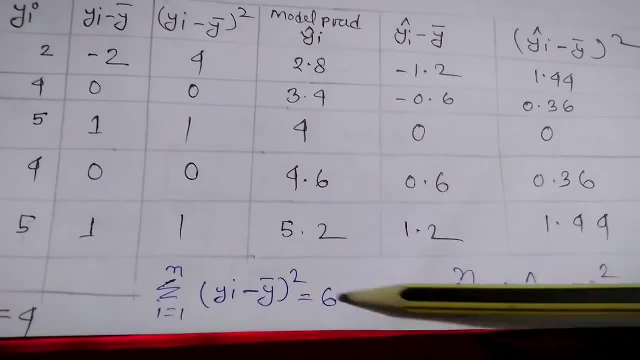 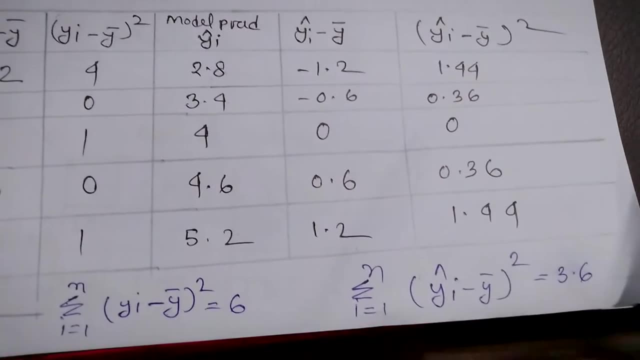 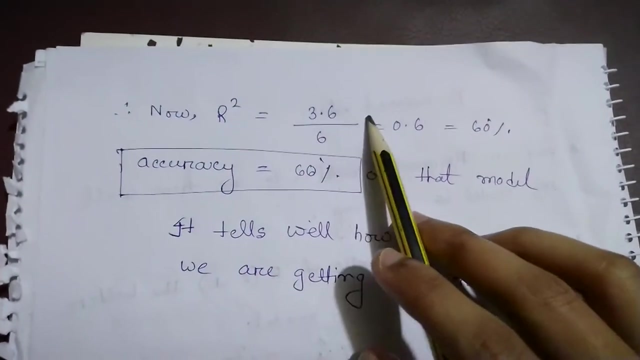 equals to 1 to up to n, y i minus y bar, whole square is equals to 6.. so our actual value difference is square is 6. our predicted values is differences square is equals to 3.6. we need to just find this ratio of it of this to this. so we get r square is equal to 3.6 divided by 6, which is actually a 0.6. 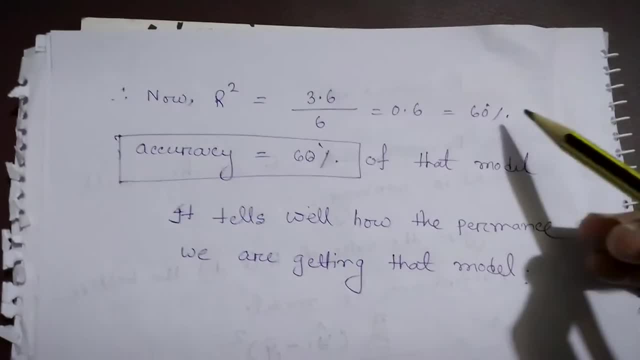 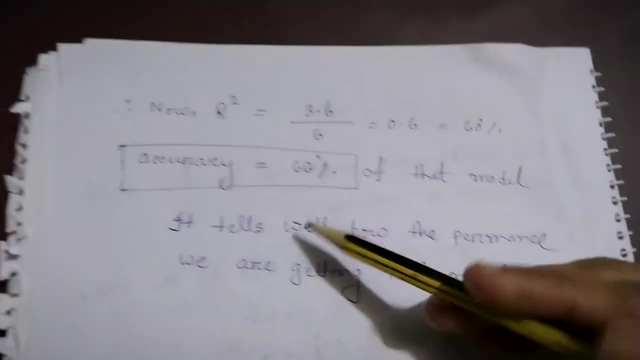 which is 60 percent. if you 100 times it, it is 60 percent accurate. so our accuracy is 60 percent of that model. it tells how well the performance we are getting from our model. the higher the output we get- uh, in upper places here, which is our predicted differences square- the more accurate. 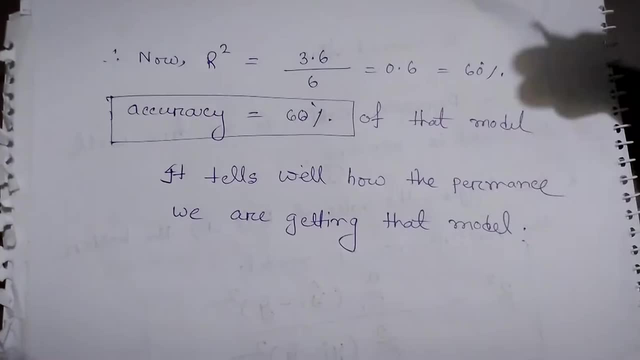 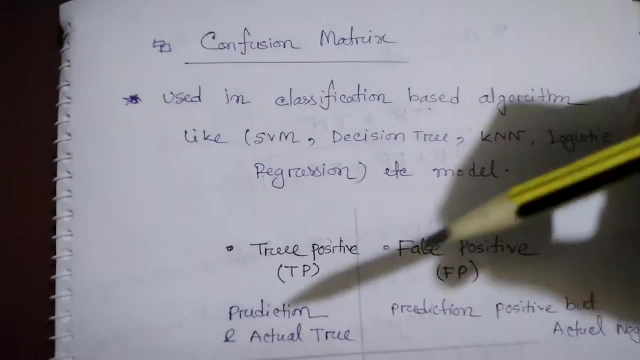 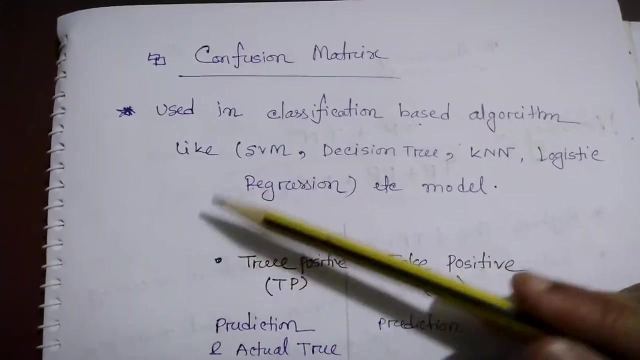 it would be and the more performance you will gain from your regression model. so, as you know, the confusion matrix is also very important. in case of you are analyzing the performance matrix of classification algorithm now, which are the classification algorithm? it is svm support vector machine that i make a video just before it just check it. also decision tree, i also make video sense and knn. 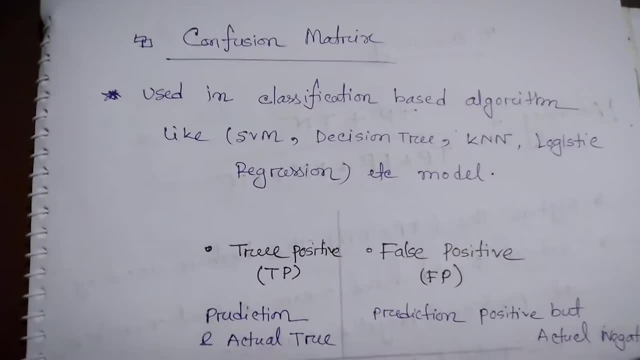 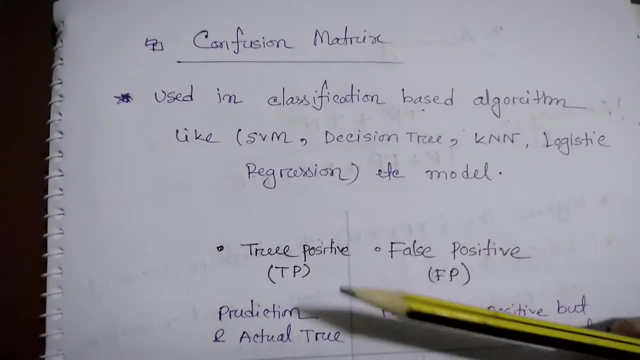 logistic regression, and all of those are classification related algorithm. also, the naive bias is also classification based algorithm, so we need to use confusion matrix to find the accuracy based on it. okay, so suppose. so let's understand. the cohort is confusion matrix. suppose we have four quadrille here. 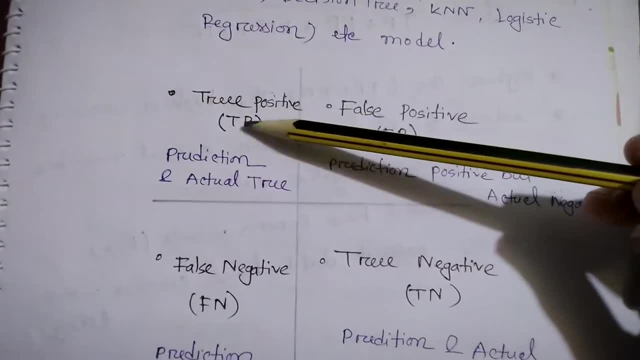 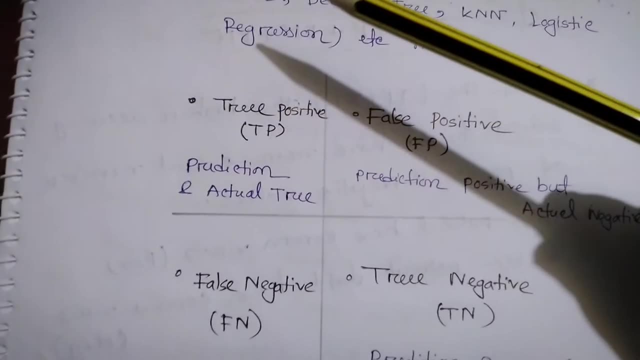 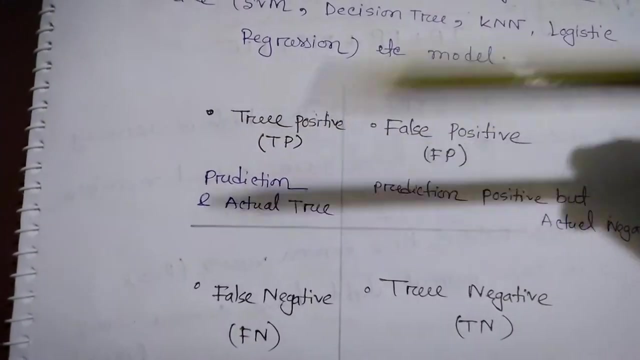 first one, we have true positive. it means that we can also say it: tp for true positive, which is prediction, and your actual value. all of them are same. true, your model predicted that you have that kind of disease, suppose cancer or any other disease, or coving 19, as you can see, and your actual value. 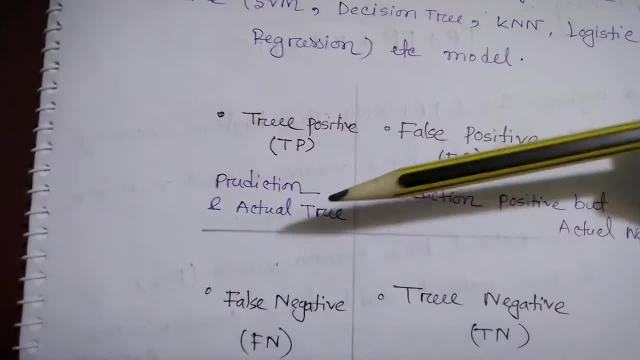 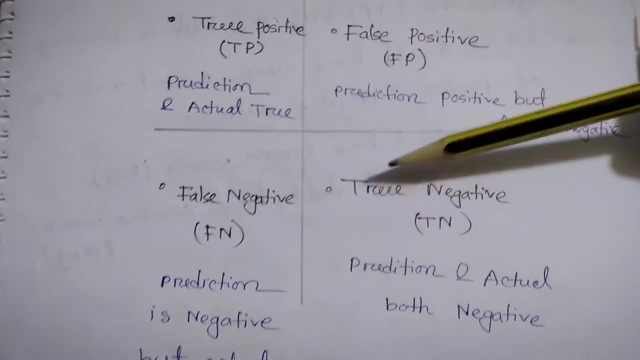 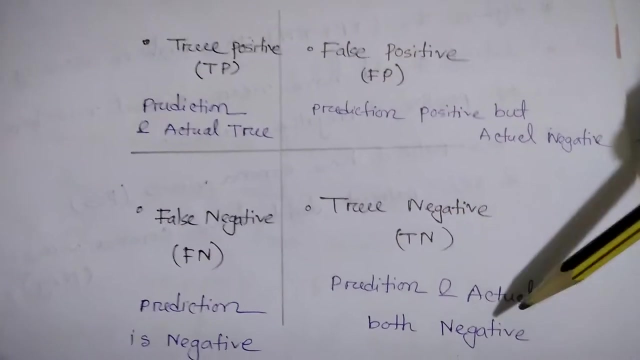 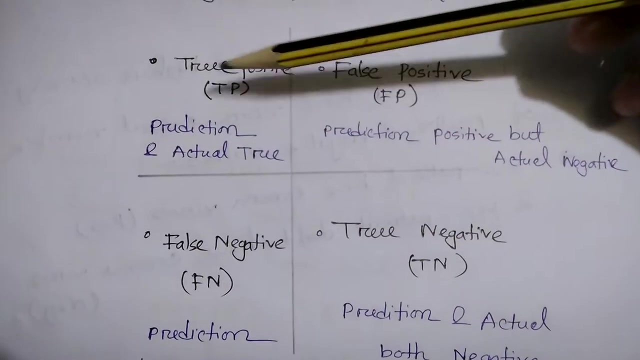 actual passion also has covered 19 and your machine learning algorithm also predicted that you have, then it is true positive. but when it is true negative, it means that your machine learning algorithm predicted you do not have coronavirus and you actually do not have coronavirus. so actual and predict are the same. then it is true negative and true positive in case of positive. 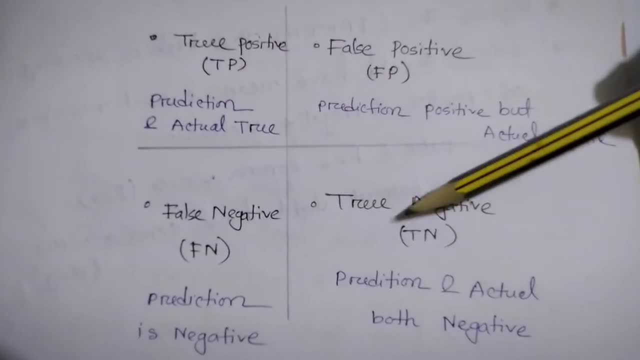 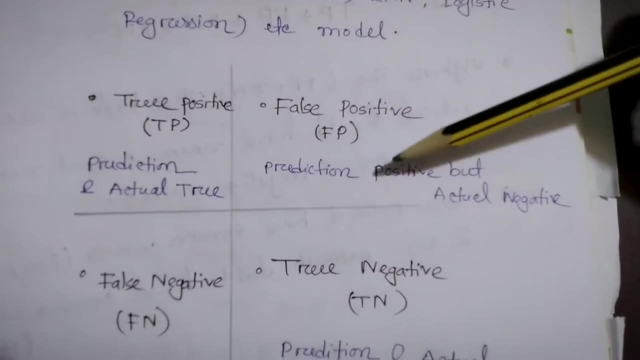 we have true positive. in case it gives negative, it is negative. this is also say tn another. we have false positive. now why it is false positive? it is actually not positive. the passion is positive. do not have actually the coronavirus, but your machine learning algorithm predicted that you have. 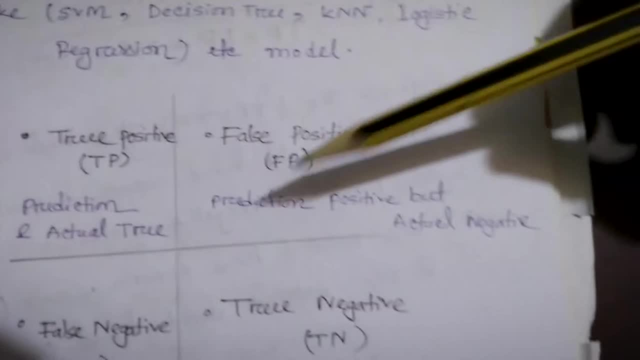 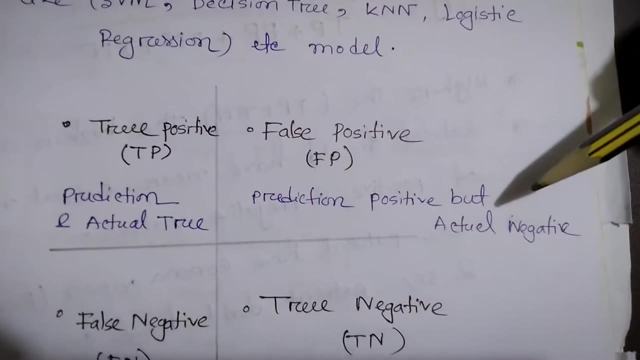 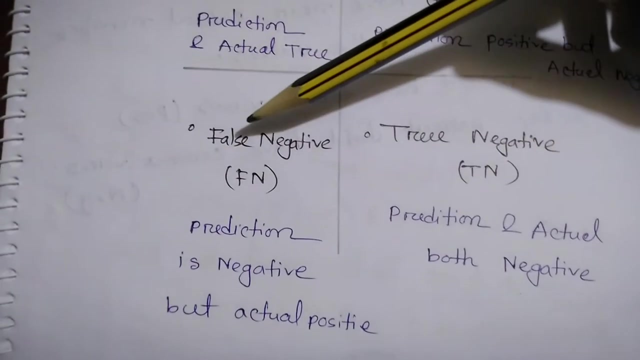 that's why it is false positive, which is FB. It says prediction is positive by the algorithm, but you actually it is a negative. actually you do not have, but in prediction you have positive. so it is false positive. Another case which is just opposite of false positive, which is false negative. 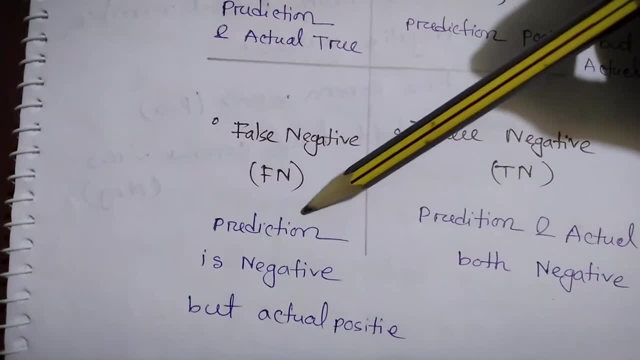 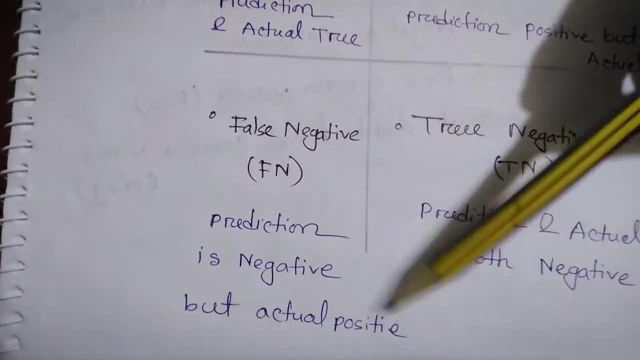 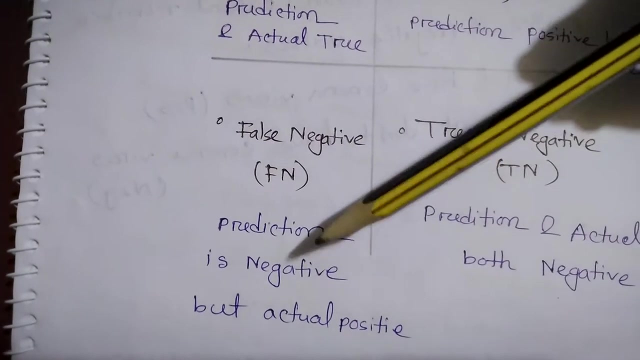 It means that your prediction is negative. your machine learning algorithm gives that you do not have coronavirus or cancer, suppose, but actually you have. actually you have, but it predicts as none. so when you case a real life scenario, there is a problem, because in it you would really have. 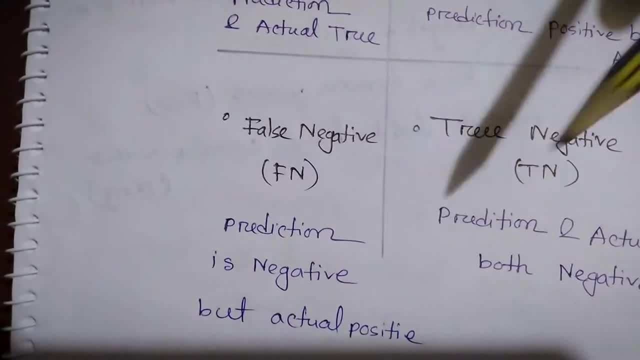 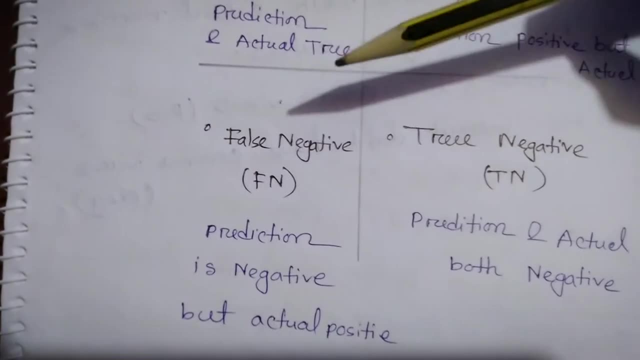 actually have coronavirus but it predicted that you do not have. so that's why there is a huge dangerous thing that if your model gives it is negative but actually you have, then it is a very dangerous thing to happen. it is disasters in analyzing this, those two things false, positive. 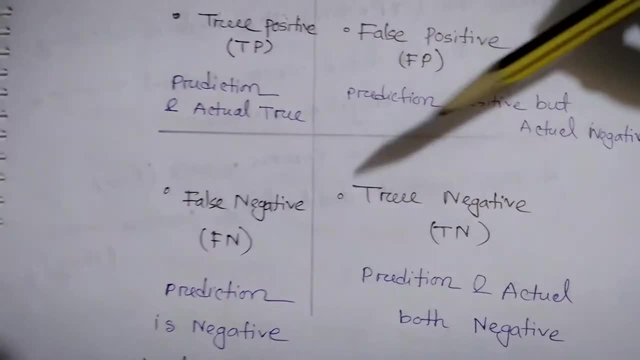 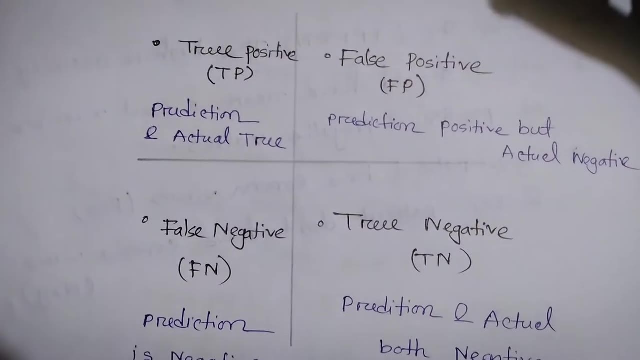 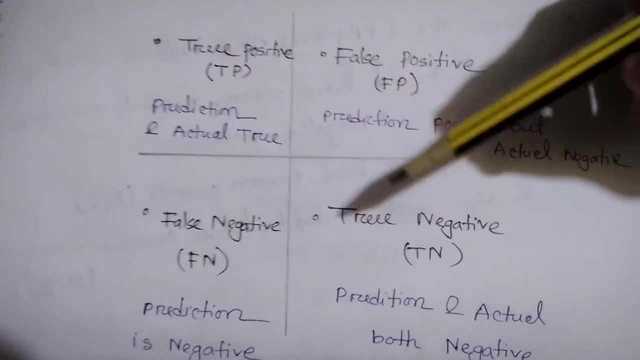 and false negative and minimize it very properly so that you get get better accuracy. and you need to understand that when the true positive and true negative are higher in your machine learning algorithm, it gives higher chances that you get better result and better performance out of those machine learning algorithms. so it is really important those true positive and true negative 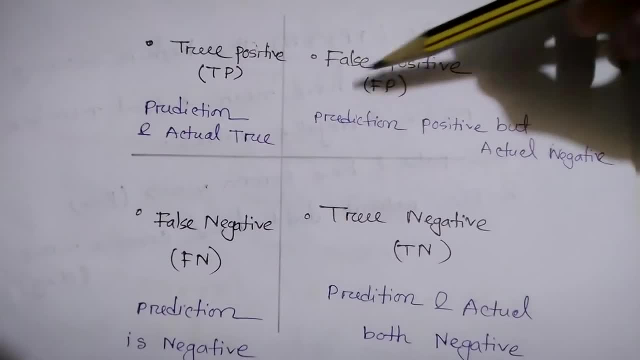 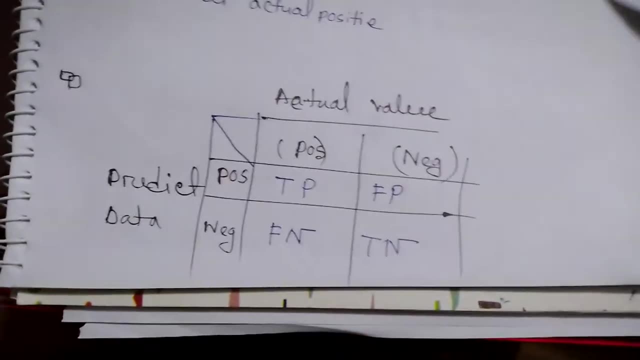 should be increased hugely. compared to the false positive and false negative. that gives very bad performance and bad very result. so you need to be really good at it, understand it. you can also understand it properly. that limits your training. you can see from paper whether it will be effective. I want to. 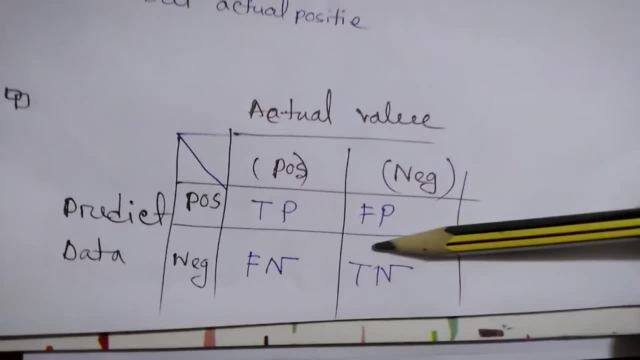 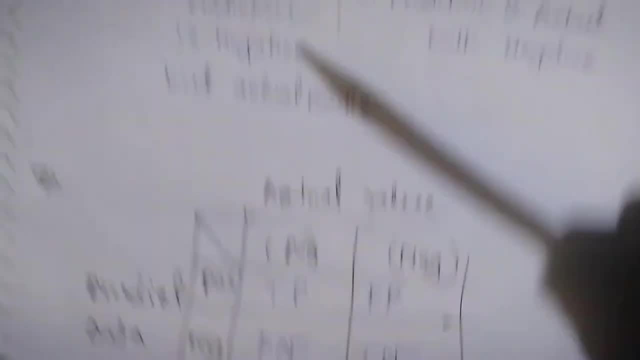 give it a good try, but if you want to surface of math classes in between, if it's not so, you can intuitively, of course you go by this diagram, where this actually a thousand positive and negative darfal one and predicted that we have a positive and negative and this tables so. 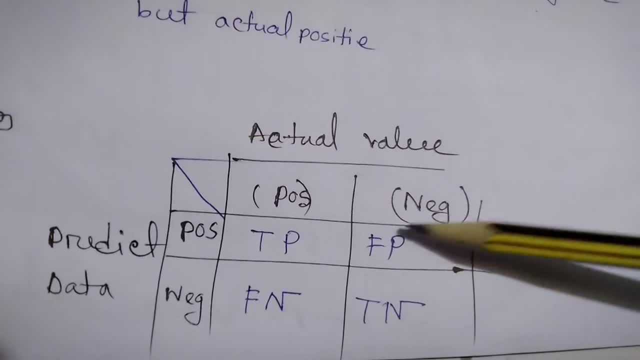 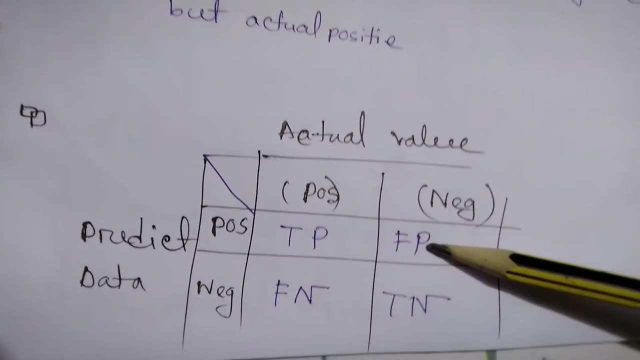 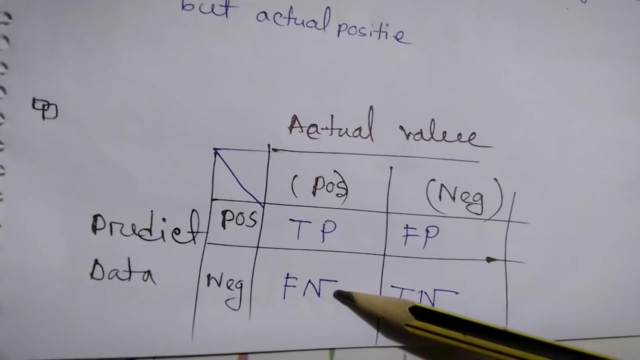 two positive here. this is super. actual value is positive and predicted values also positive. so we have true positive, which is this one, so bottom them are positive. so it is false positive. another is false negative. it means that actually you have those disease okay, but your predicted data is negative. but you actually have positive, but you predict it. 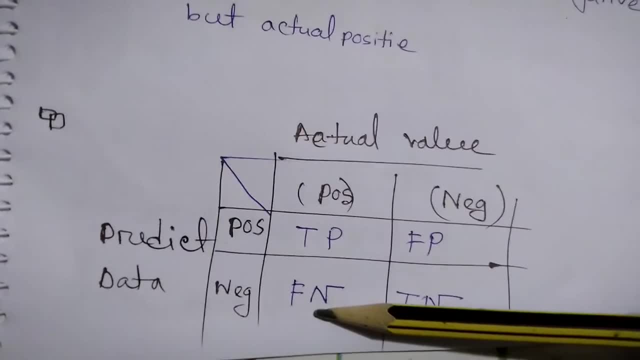 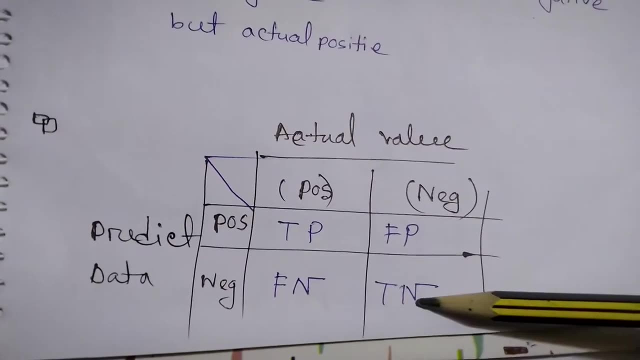 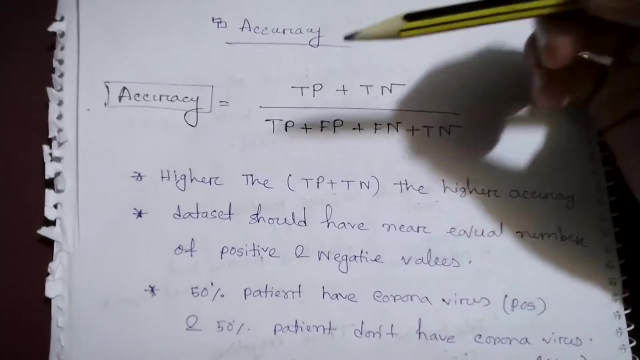 is negative, so it is false negative. you have positive, but it predicted need and true negative when your actual value is also negative. predicted data is also negative. it is true negative. simple as it is based on your confusion matrix. we get different kind of formulas, different kind of. 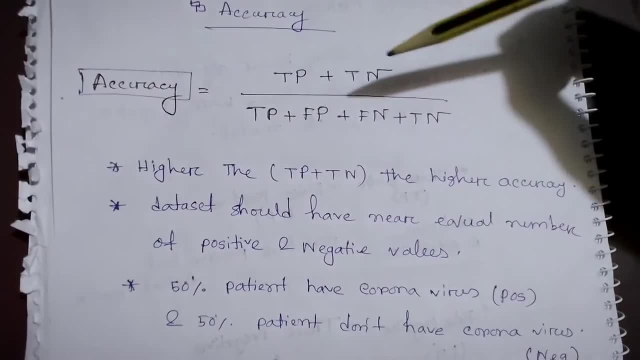 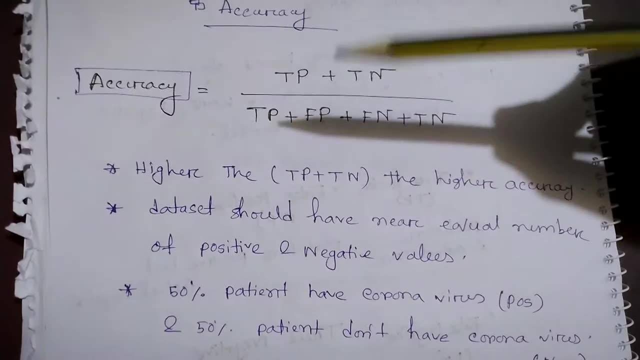 equation. to find the accuracy- though our accuracy is- the equation is true positive plus true negative- we need to increase their sum divided by total outcome. total outcome is true positive, false positive, false negative and true negative. so these are the total outcome and then sum, and in the upper 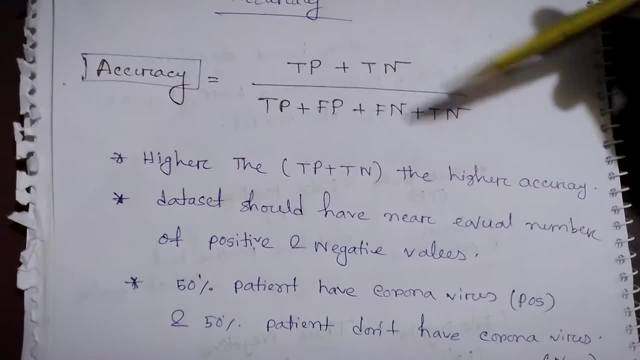 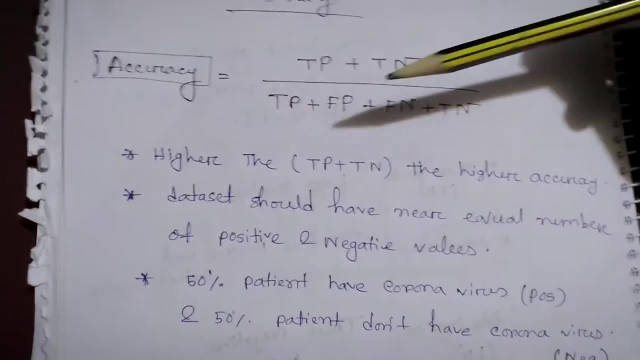 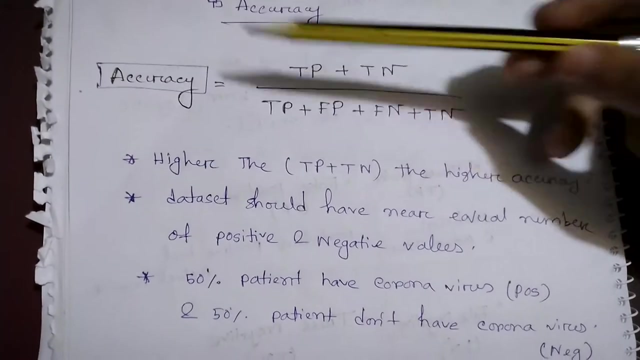 case we have on the upper side, we have on the true positive and true negative. when the true positive and true negative are higher chances and is higher in this mathematics, it means that your accuracy is higher. according to this equation, your accuracy is higher because when your upper side increases, your accuracy also increases when your lower side. 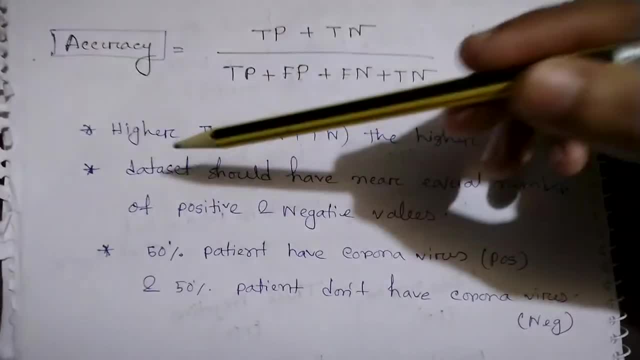 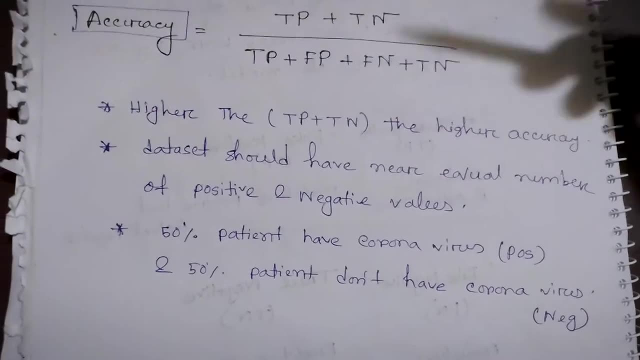 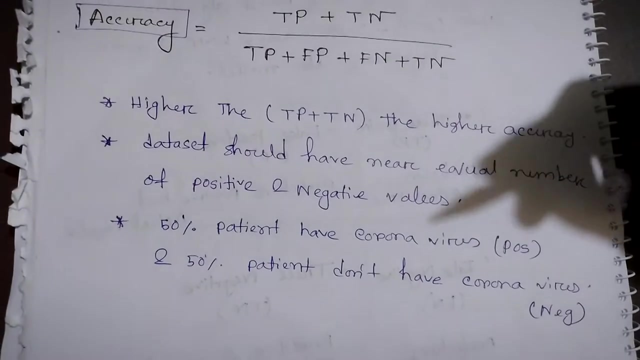 this increases. it means that your accuracy falls down. so your data set should have near equal number of positive and negative values. it means that suppose in you know, in your training data set you have only 20 people or 5 people who have cancer, but 95 of them don't have cancer. so when 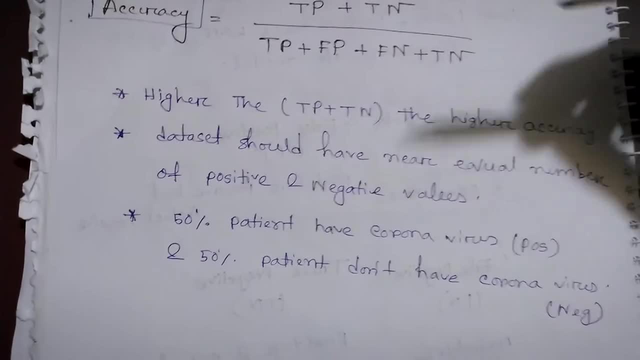 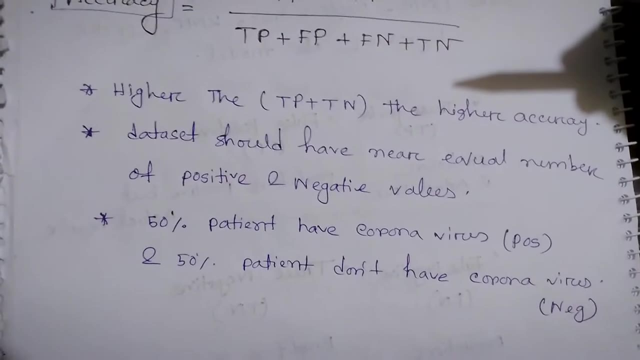 you run your data, you can macro, tengo it and then set a set of 3 or 4 gaps of your chemistry to increase that model. it always gives that you do not have cancer, because there is only five percent people who have cancer but 95 of them don't have. so your prediction will always go to the 95. you don't say. 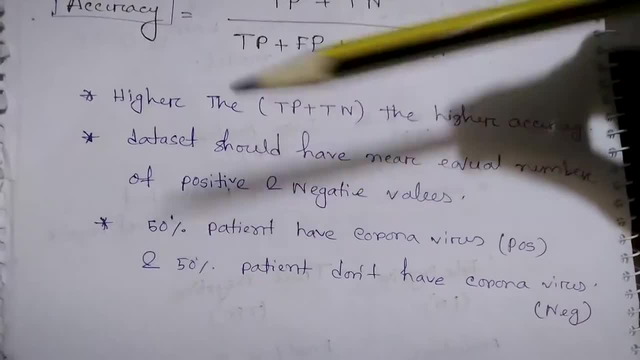 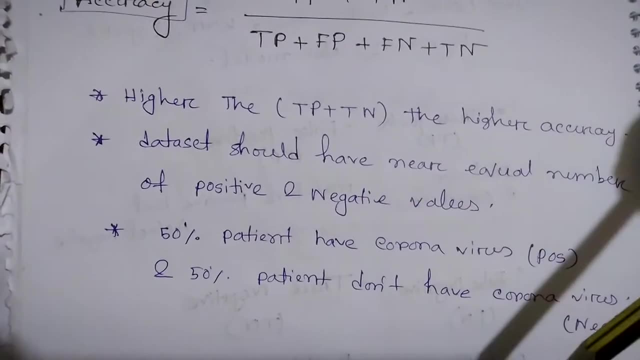 that you do not have cancer, but actually you will have. so this is a big problem. so you should always use equal number of data set: 50 percent of the people should have cancer and 50 percent of them should not have cancer, so that your model understand it properly. so you need to give 50. 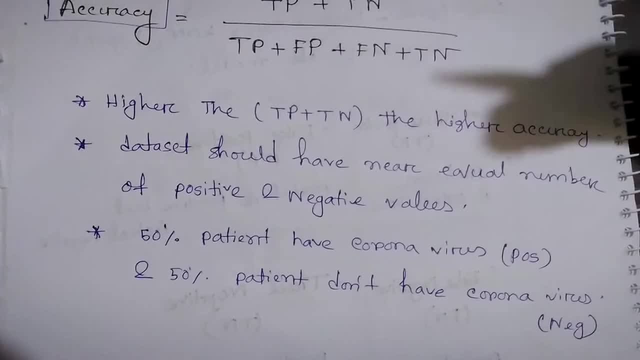 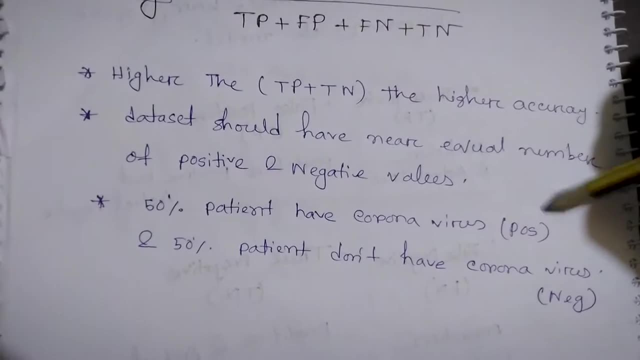 50 percent chance of your near 50, 50 percent of your chance of a training data set so that you get better accuracy. so it says 50 percent of the patient should have coronavirus positive and 50 percent of the patient don't have coronavirus negative. so your data set should be in balance. 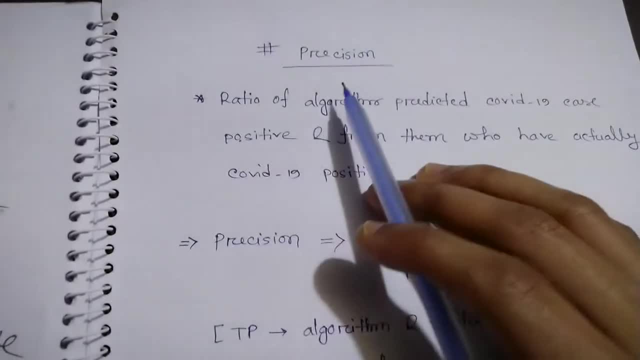 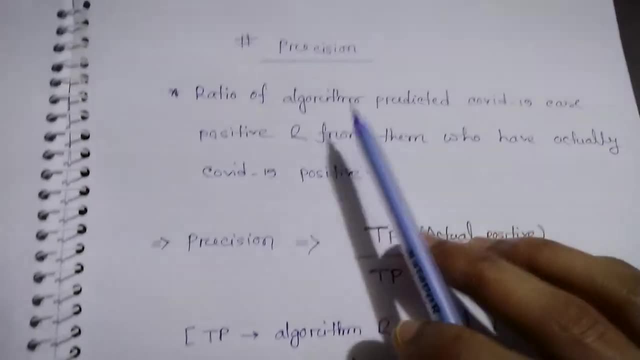 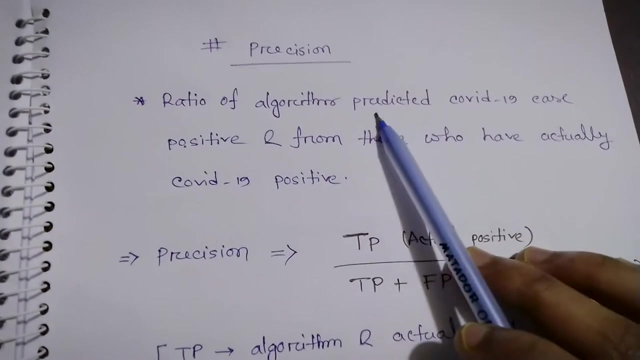 so that you get better output and better accuracy. let's see what is precision. it is very important to understand, so please concentrate on this. so precision is actually the ratio of algorithm predicted covid 19 case or any disease, suppose cancer or any other case, the algorithm predicted covid-19 case positive, and from them who have 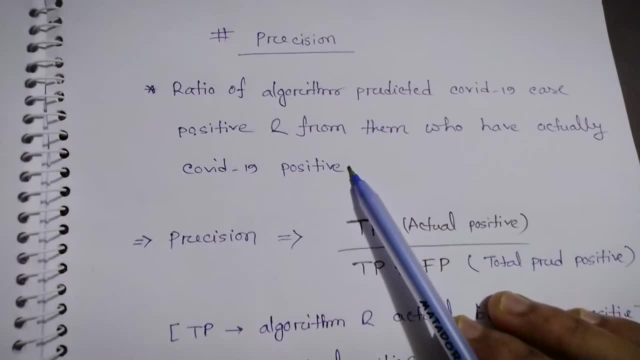 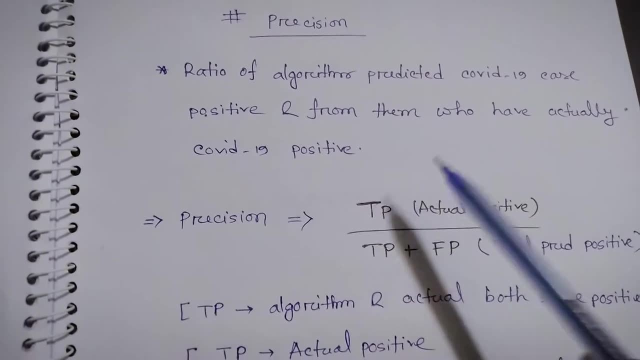 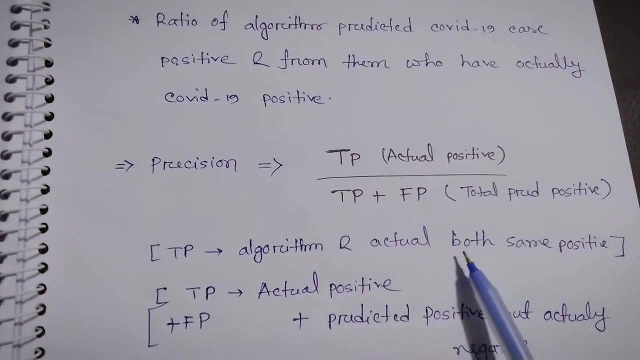 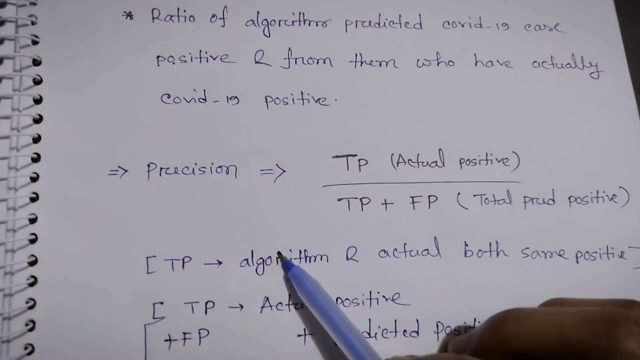 actually covid-19 positive. so from the confusion matrix you know that the true positive, which is actual, positive and algorithm predicted positive, so it is the same. so true positive is actually the algorithm and actual, both are positive. so it is covid19 positive case, which is also predicted by algorithm and also in real life. okay, so it says: 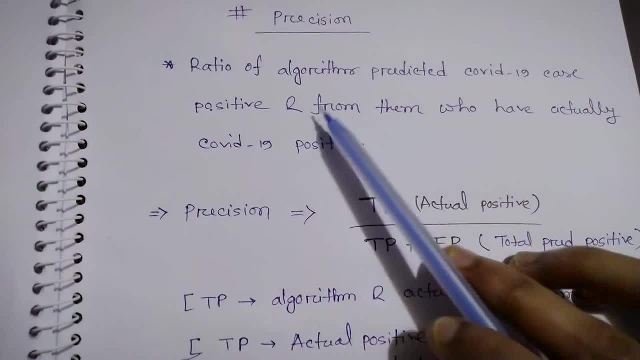 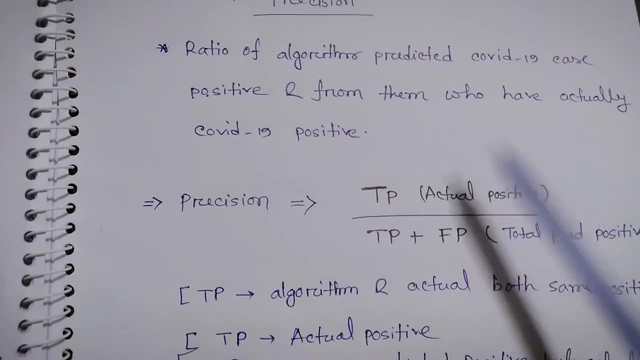 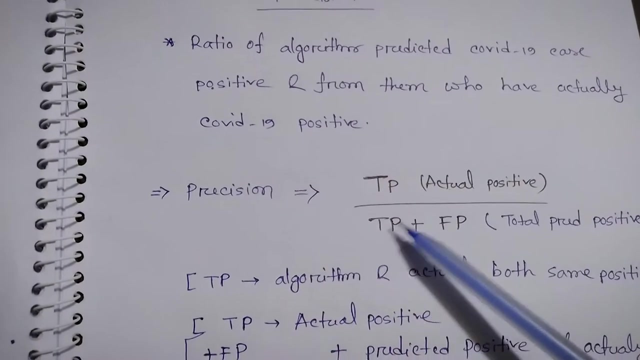 the ratio of algorithm predicted covid19 case and from them who have actually covid19 positive case. so tp is the actual positive covid19 case divided by total predicted positive case by the algorithm, which is true positive plus false positive. now what is false positive? false positive is actually. 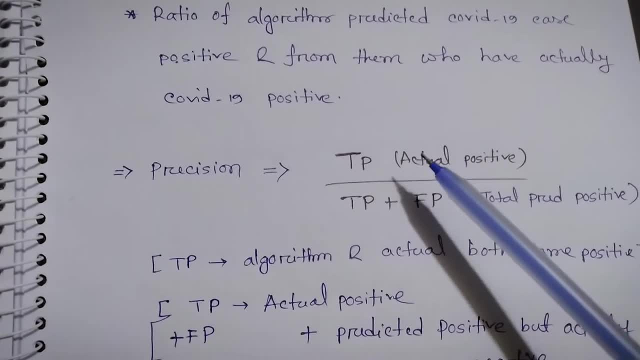 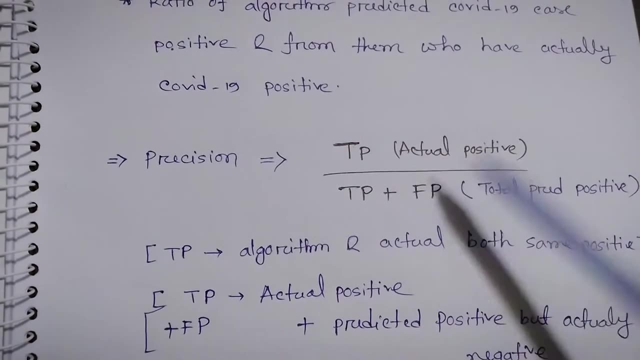 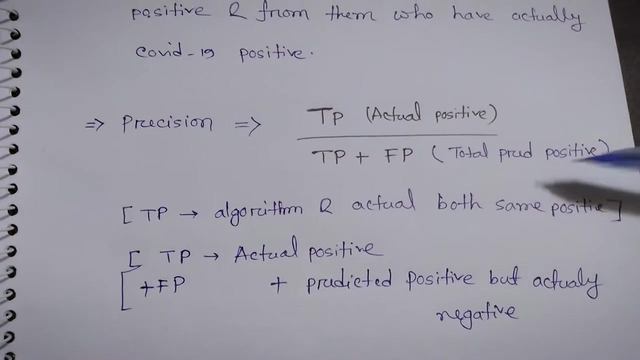 which is predicted as positive by the algorithm, but actually you do not have covid19 positive case, so this is actually a negative thing. okay, the false positive- so let's see tp is actually. both of them are positive, algorithm predicted positive case and actually positive and in the lower side. 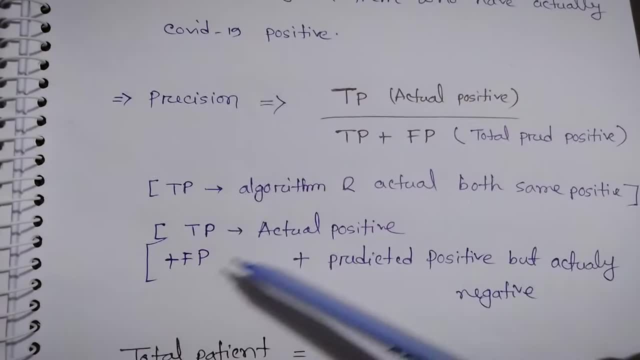 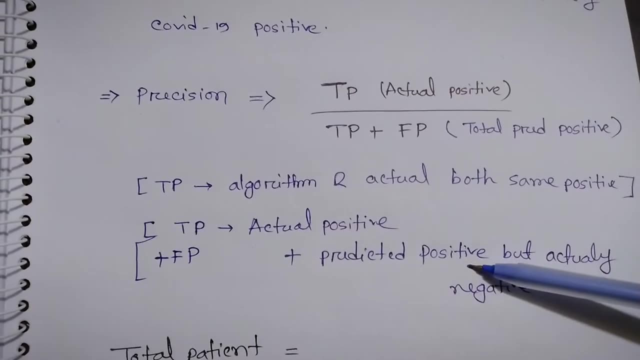 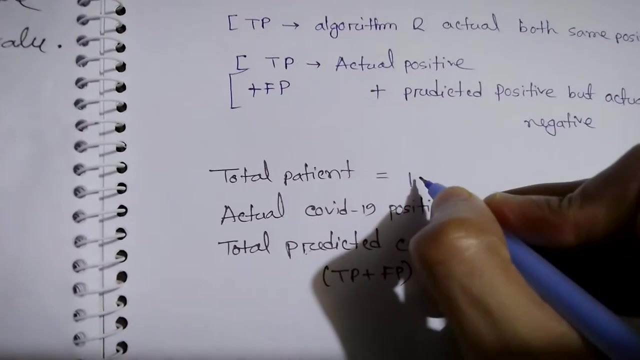 we have tp plus fp, which is true positive plus false positive. true positive is the actual positive case and false positive is the predicted positive case by the algorithm. but actually you do not have, actually it is negative. so their ratio. so suppose we have 100 patients total patients, from them actual covid19 positive 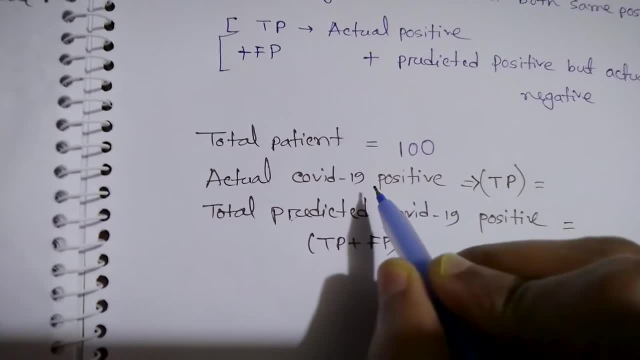 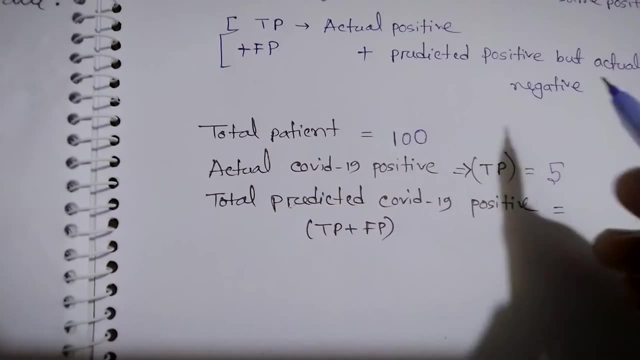 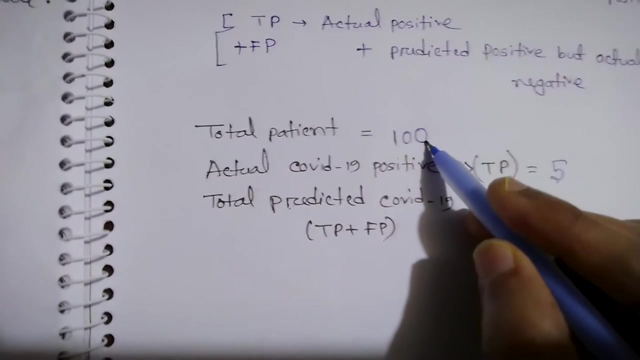 case by the algorithm predicted positive and actually positive is only five. so true positive is only five. so and the total predicted covenanting positive case by the algorithm is true positive plus false positive. so total is 100 patients. five is actually positive and the tp is actually the five plus. 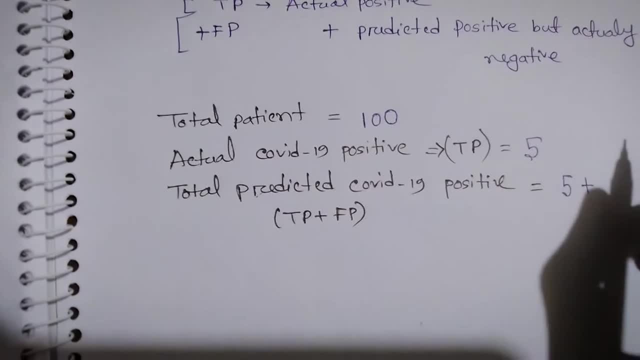 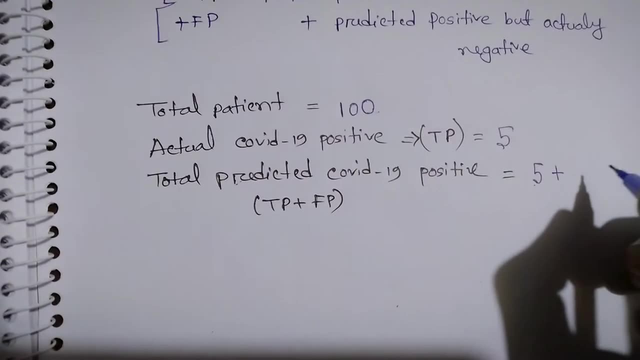 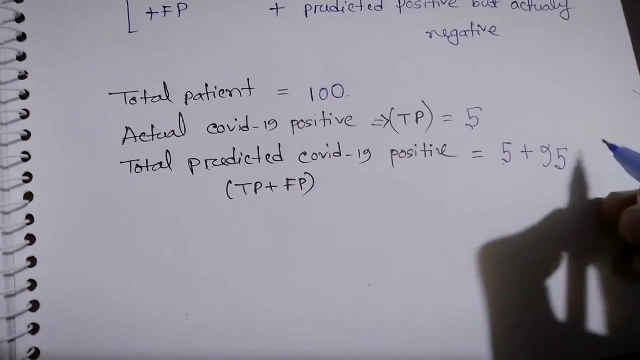 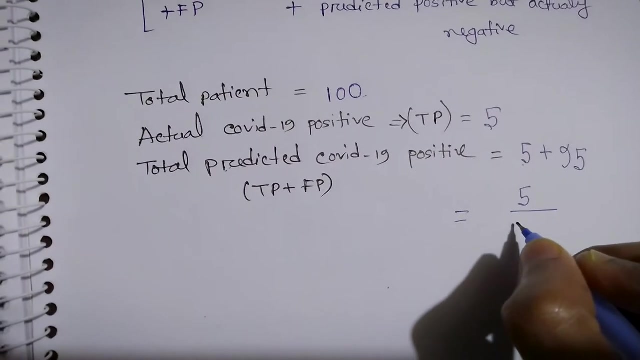 fp is the false positive algorithm predicted as positive, but actually they do not have coming in, so only five of them has covenanted. so 100 minus five is 95.. so they do not have copy 19, but the algorithm predicted as positive. so total is 100. okay, so tp is 5 divided by tp plus. 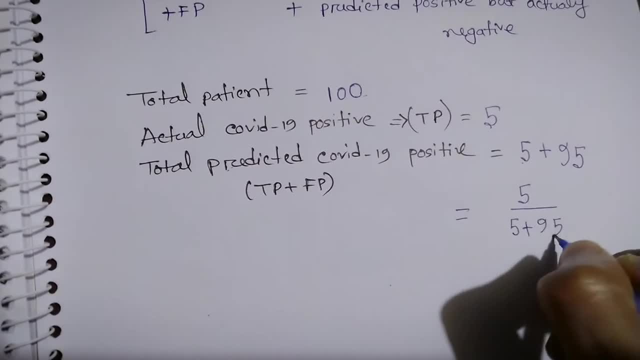 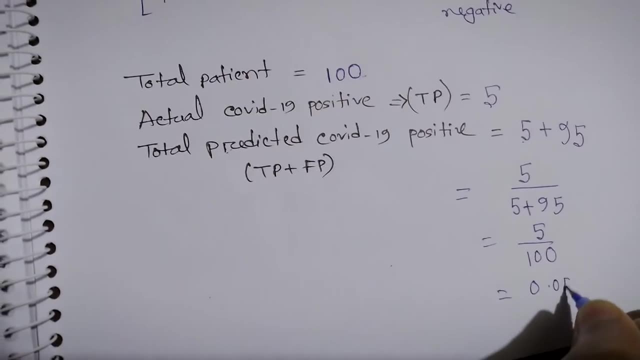 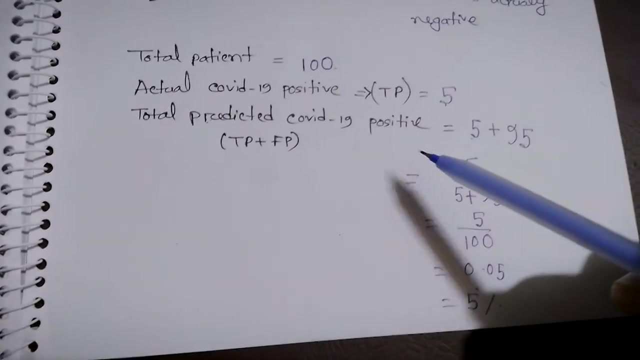 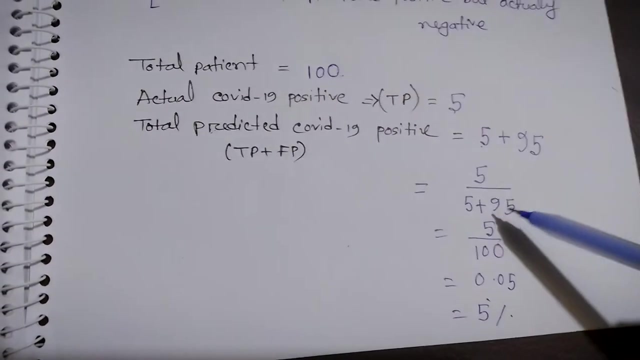 fp, which is 5 plus 95. so 5 divided by 100, which is, you can say, 0.05 or 5, so your model accuracy is only five percent by given in this kind of scenario, when five of them has actual covenanting and predicted that total 5 plus 95, which is false. 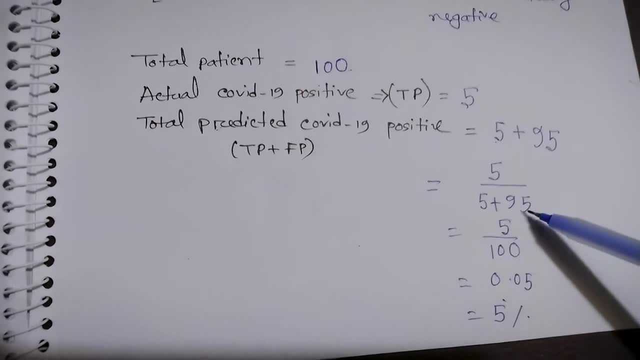 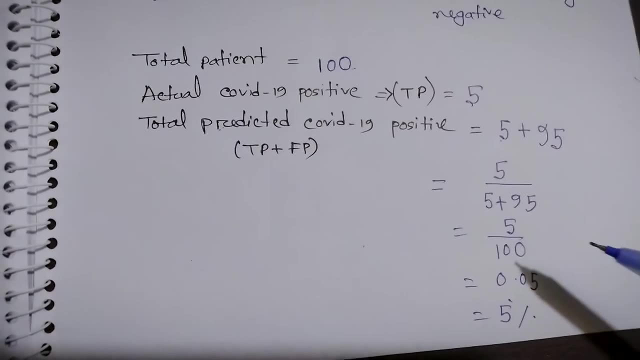 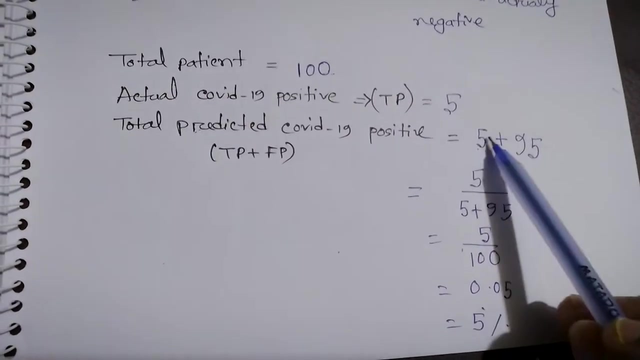 positive. they do not have covenanting, but the algorithm predicted they have covenanting, so it is 95, but actually they do not have covenanting. so false positive is negative thing. if there is total 10 operations who have actually covenanting out of 100, then 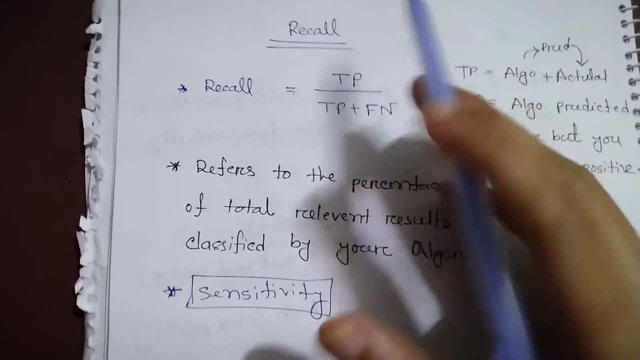 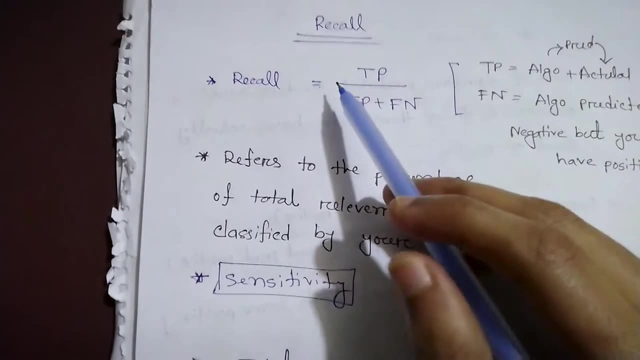 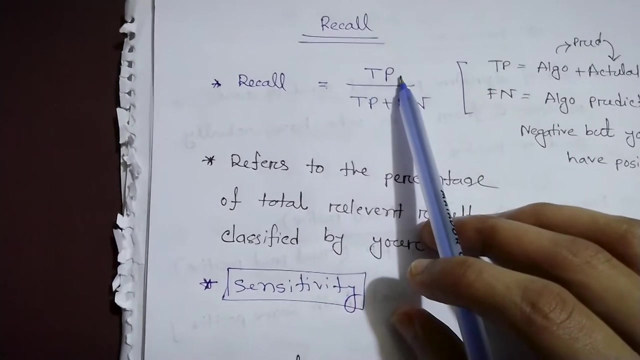 it would be 10. so let's understand recall, which is another part of your performance matrix, of your machine learning algorithm, especially in classification. so recall is actually almost same as precision, but it is more precise. recall is actually the true positive or the predicted as true positive case for covenanting true positive. 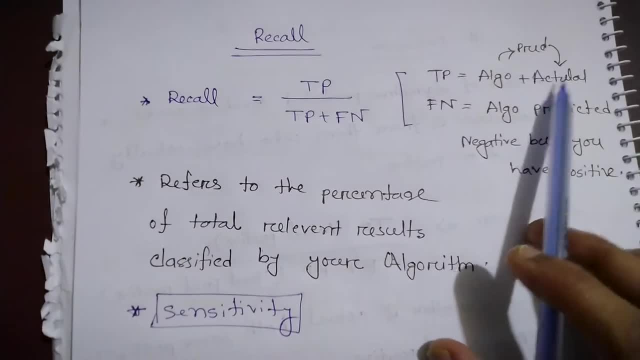 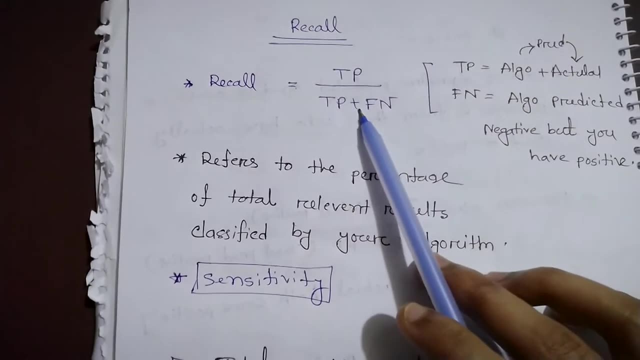 actually is the true positive case for covenanting. so recall is actually the true positive. as actually you know, the algorithm predicted positive and actually positive. so you can say the algorithm predicted actual positive is true positive and divided by the true positive plus false negative, true positive is again the same and false negative is actually the algorithm. 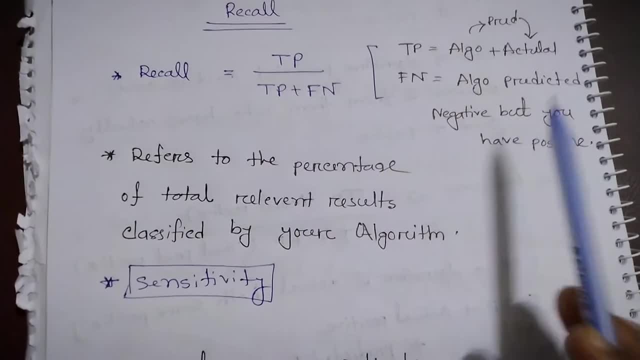 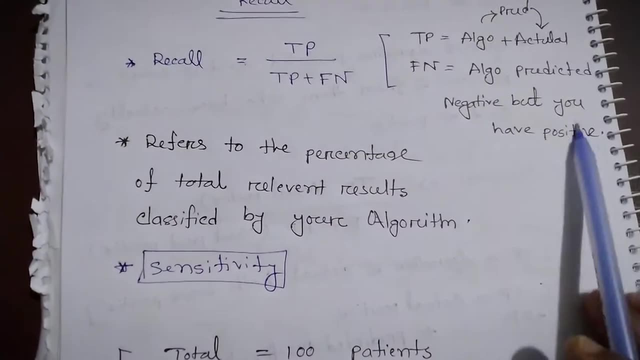 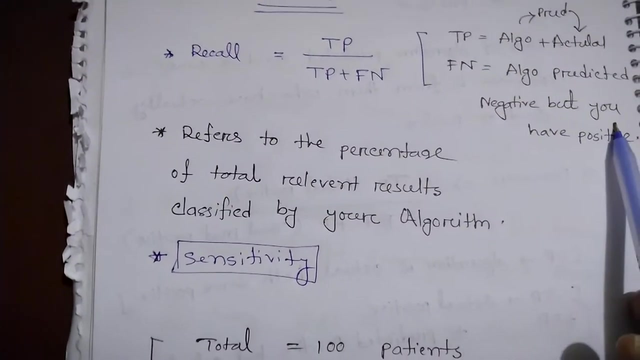 predicted as negative that you do not have copy 19 case, but actually you have positive. so false negative is actually an actual positive thing. it is negative in case that your algorithm predicted negative, but actually you have positive in real life. so this is actually the false negative- this. 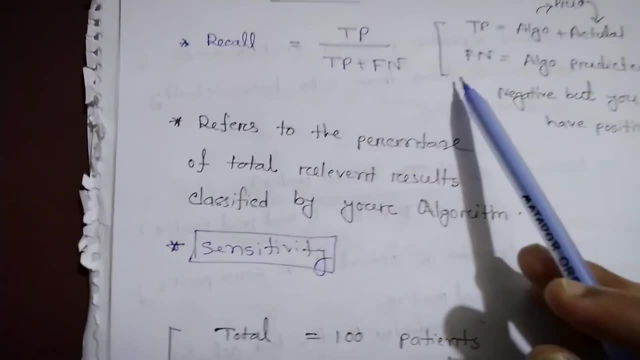 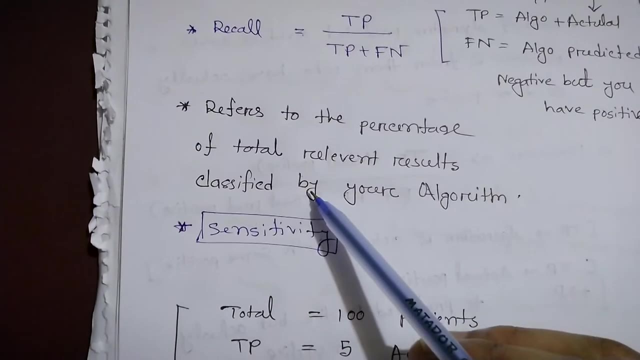 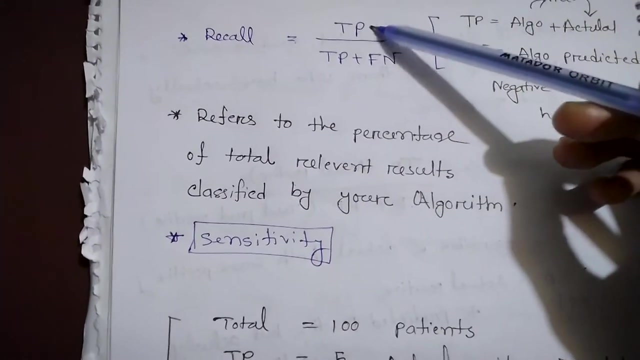 is same as the concept of confusion matrix that i have talked before, so let's see what it means. it refers to the percentage of total relevant result classified by your algorithm. so, total relevant result: what are the positive cases we are finding out of total actual values? okay, so this is our actual values that we have. 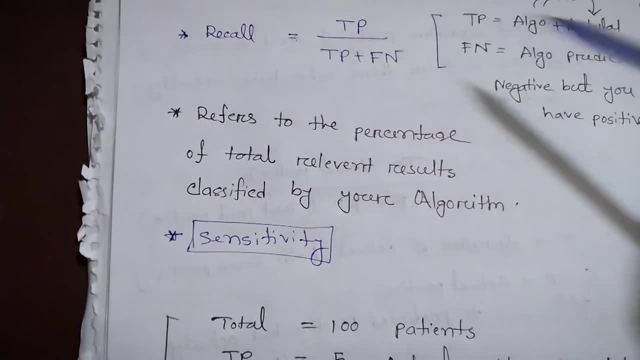 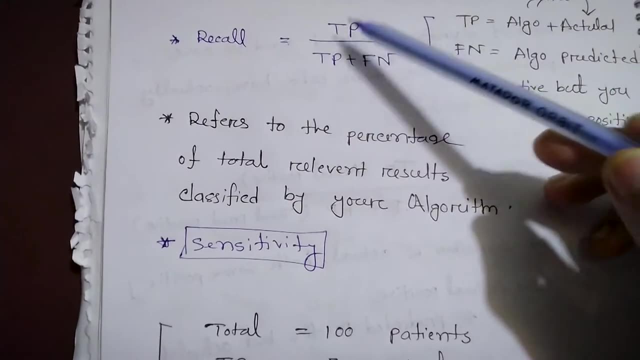 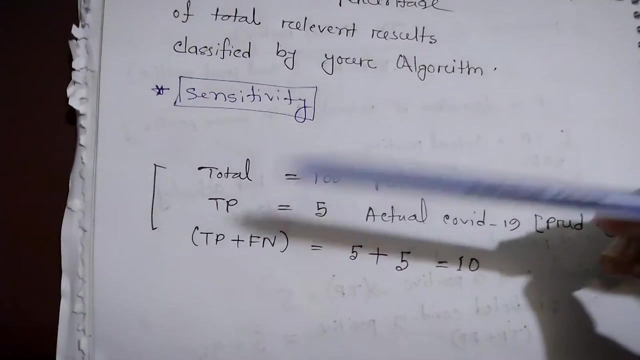 copy 19 case predicted true and false. negative is actually a positive thing that you actually have copy 19. so out of this, how many actually predicted true by your algorithm? so this is also known as sensitivity in many cases. so let's say our actual cases, suppose total, we have 100 passions. 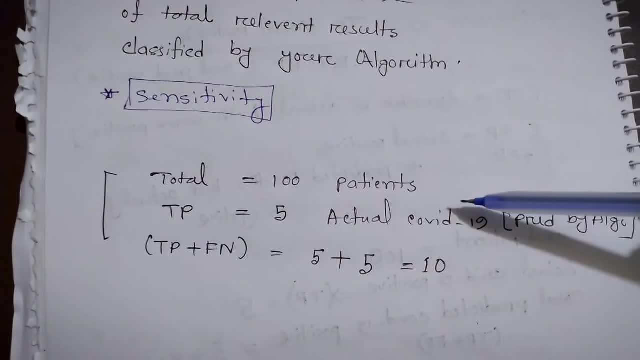 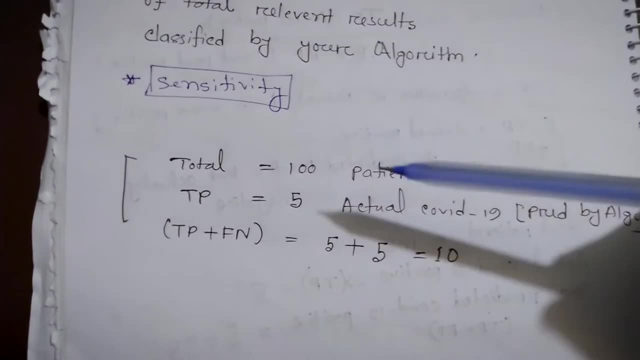 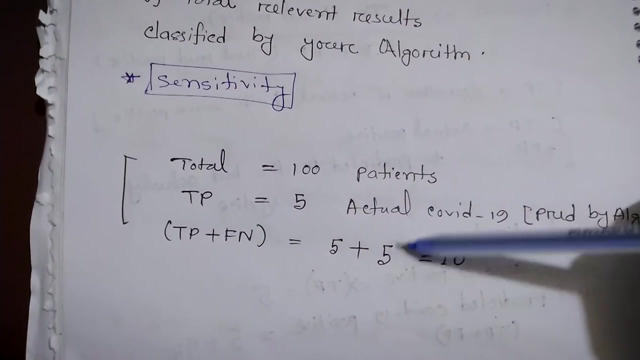 true positive, which is 5, which is actually positive, which is also actually predicted by your algorithm. that five of them has actually covenanting case. so five divided by true positive is actually the five. false negative is actually a positive thing that we only have five of them actually. 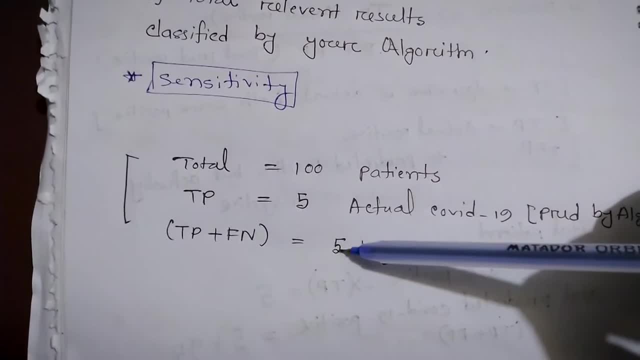 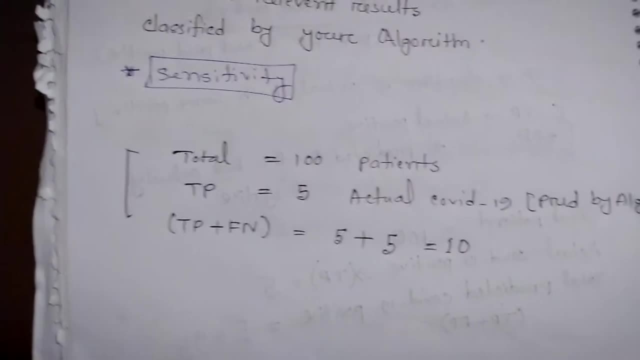 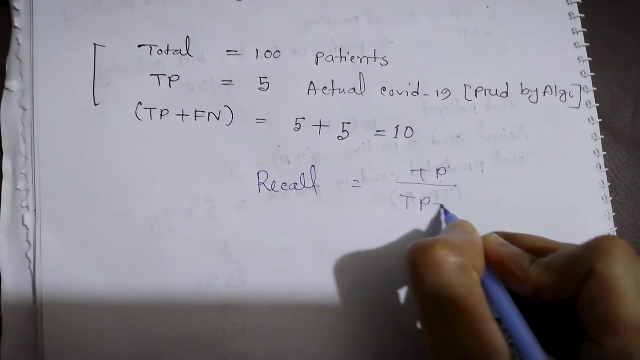 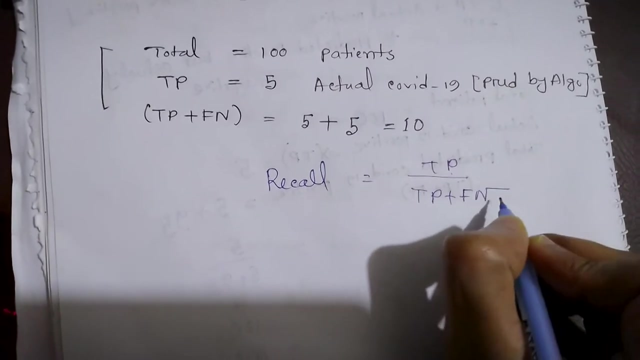 has covenanting case and the total predicted is five. so just add them: true, positive plus false negative, so total is 10. so we can find the recall: true positive divided by true positive plus false negative, which is actually the true. actually true, but your algorithm predicted false. so 5 divided by 5 plus. 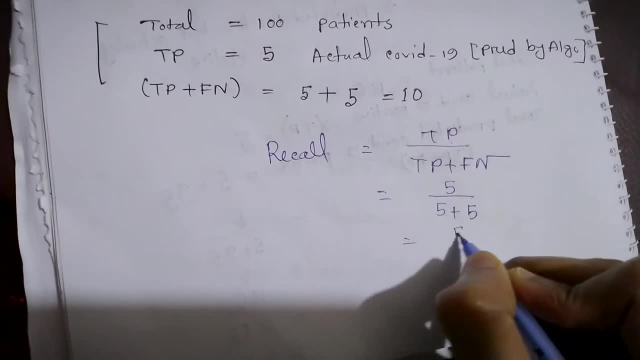 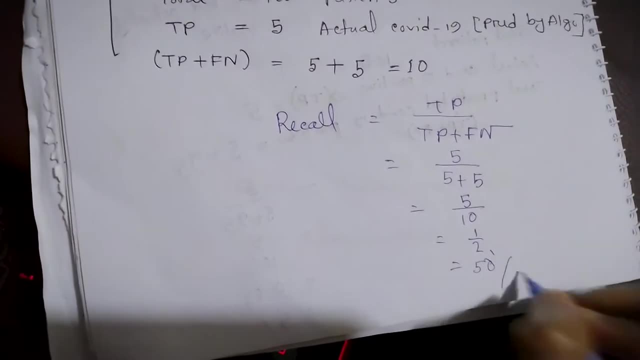 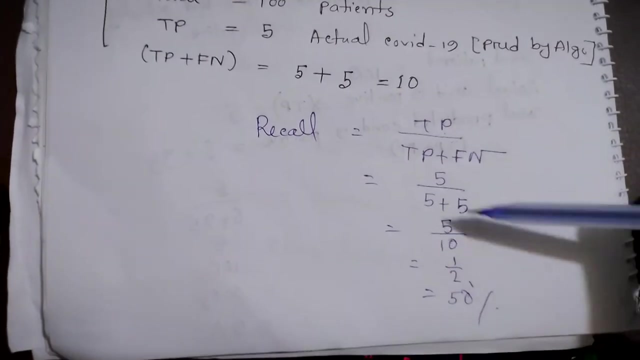 false negative is actually 5. so total is 5 divided by 10, which is half. it means that 50% accuracy of your recall in recall you get 50% accuracy here, but precision we get only 5%. so there is another algorithm or another technique. 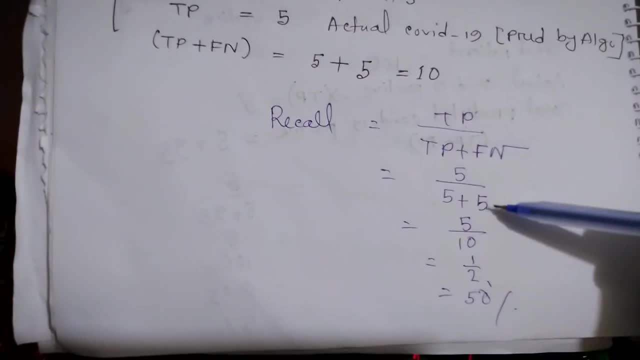 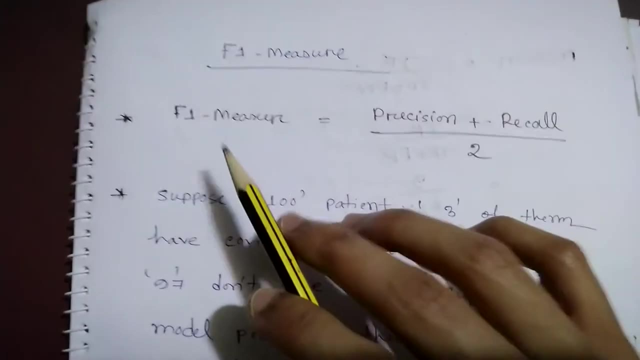 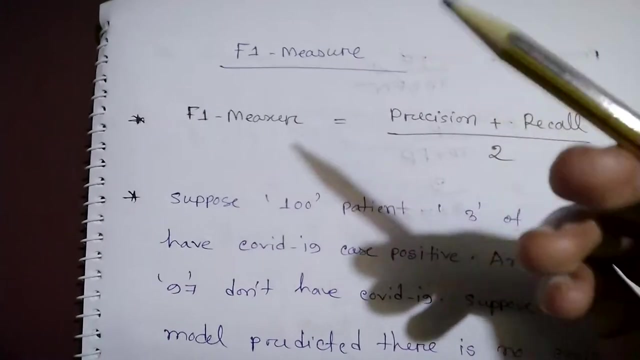 that you can find a better result, which in which is F1 measure that combines precision. recall both of them. so let's understand. this is now. let's understand the F1 measure, because it punishes this algorithm very badly and it is one of the most perfect technique to find the result: how many percent it is correct. 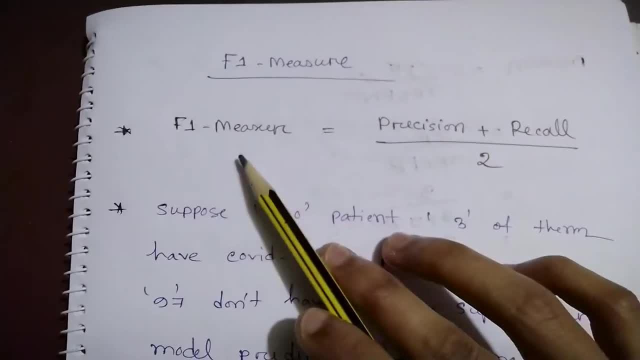 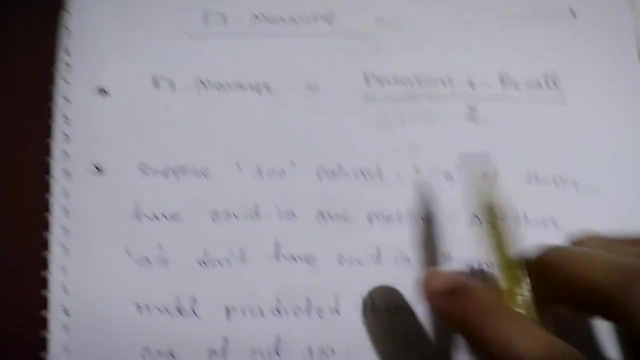 and how correct it is. so F1 measure is the. so the formula for F1 measure is precision plus recall divided by true. you just find the precision plus recall. you just find the precision plus recall divided by true precision and recall from the table and divided by simple, suppose we have 100. 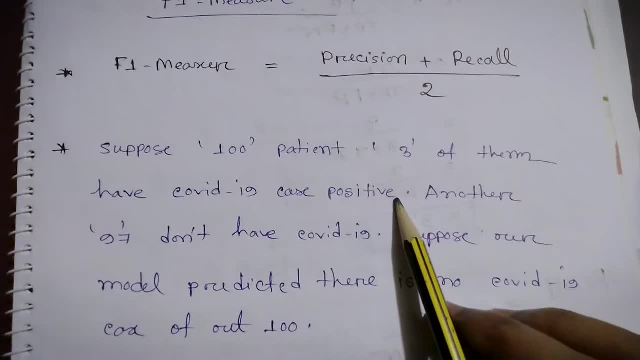 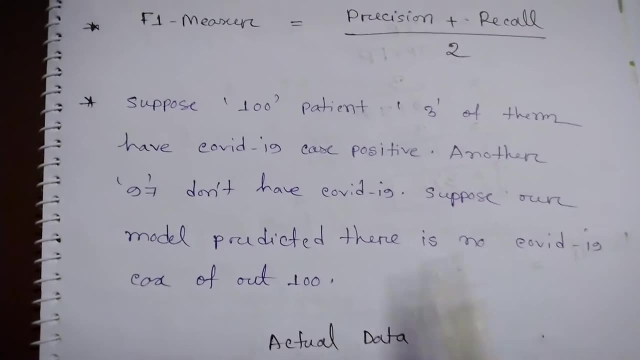 patients and three of them have COVID-19. case positive: okay. another 97 of them don't have COVID-19. suppose our model predicted that there is no COVID-19 case out of hundred? okay, because there is. only three of them has COVID-19. but 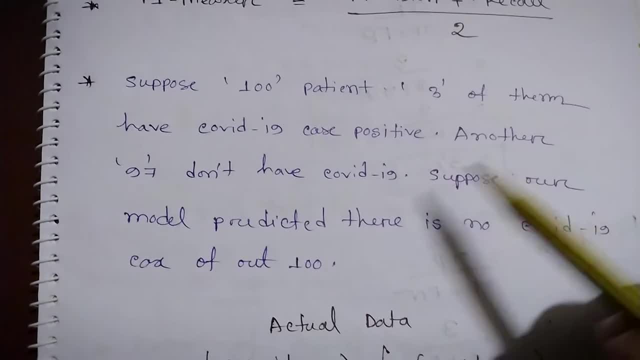 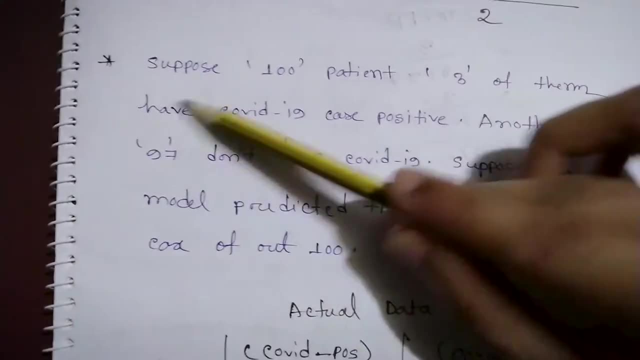 90% of them don't have. so our model definitely predict that there is no COVID-19 patient because only 3% actually have but 97 of them don't have. so it will obviously come here with 97, we will go and do the 97 it will support. 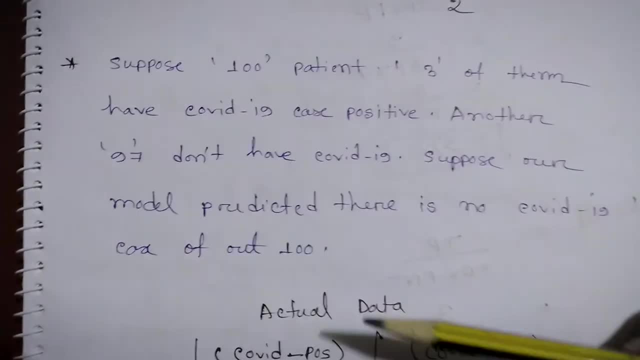 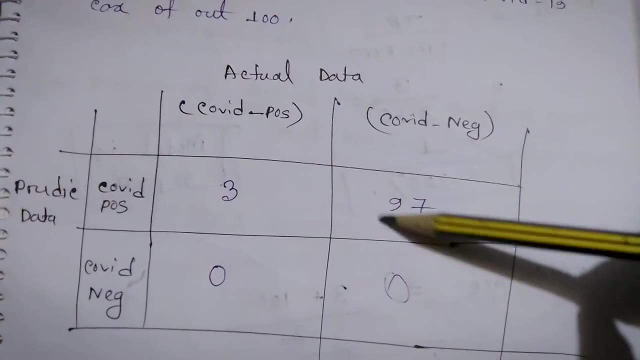 97, because the 97 don't have COVID-19. so we will predict it does not have COVID-19. so suppose our actual data is suppose COVID positive and COVID negative. three of them has actually COVID-19. ninety of ninety, seven of them don't. 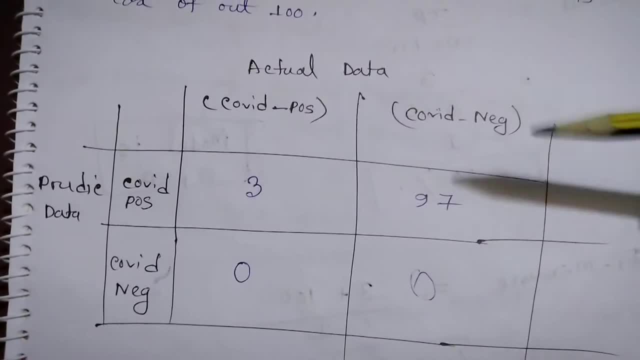 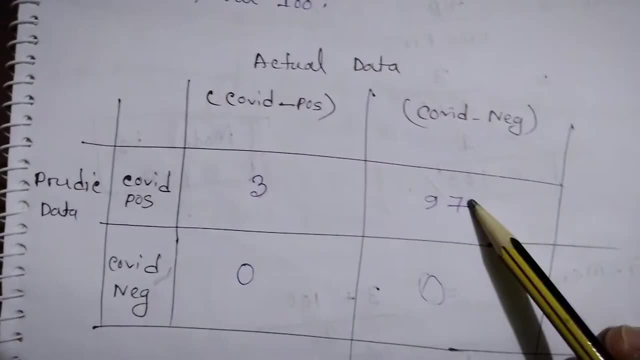 have COVID-19 at all and suppose our prediction data is positive and negative. suppose we predicted a positive is 3 and negative is 97- okay, this is your model, etc. and negative is 97- okay, and other cases suppose zero. zero because it can only predict when there. 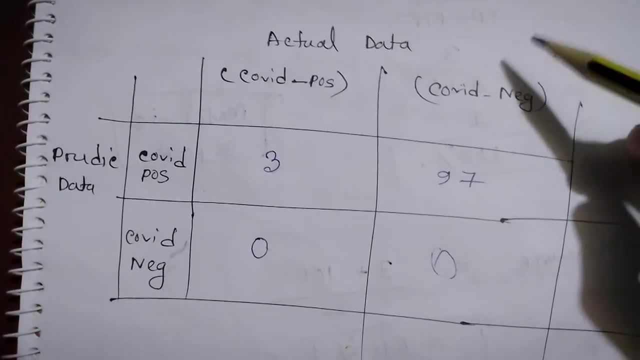 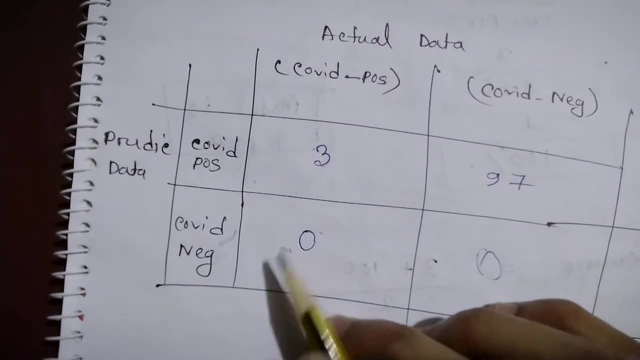 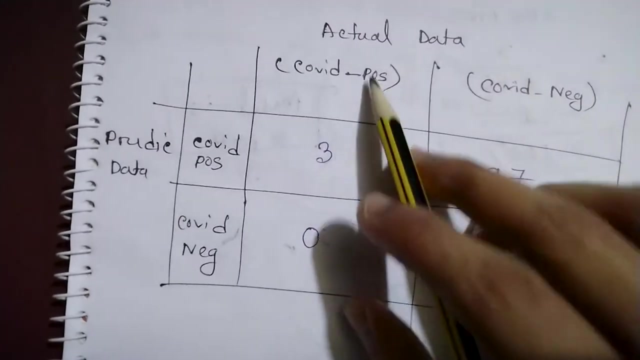 is no copy. 19, your model is not trained perfectly. your actual is zero. your prediction is also negative- is zero. it says there is no negative case- okay, when you're actually having three positive, but it says there is no positive, so it is really bad condition. and when it says the 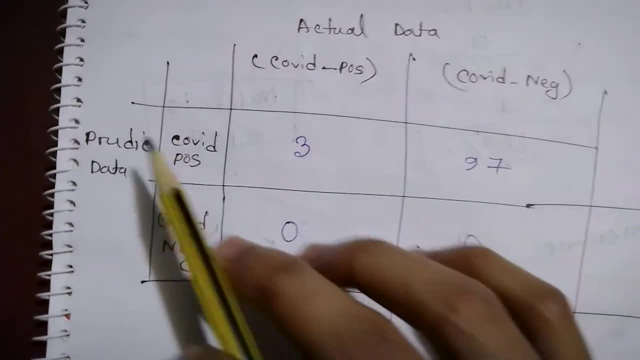 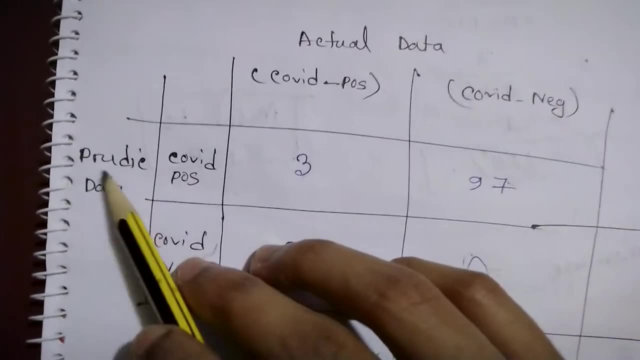 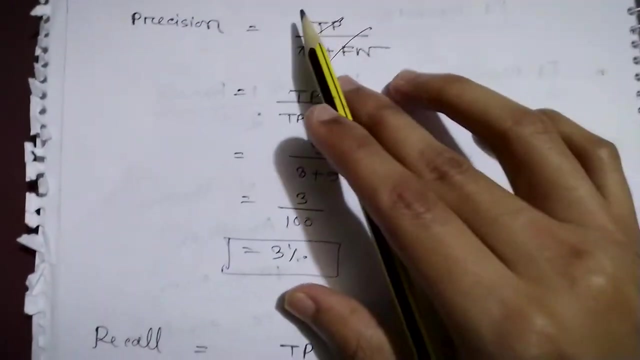 negative is total 97, but your prediction data said you have copy 19, but actually you do not have copy 19, but predicted model says yes, you have 90 of them. okay, so your model is not that good precision. say so to understand. you need to find precision and recall so that you can find f1. 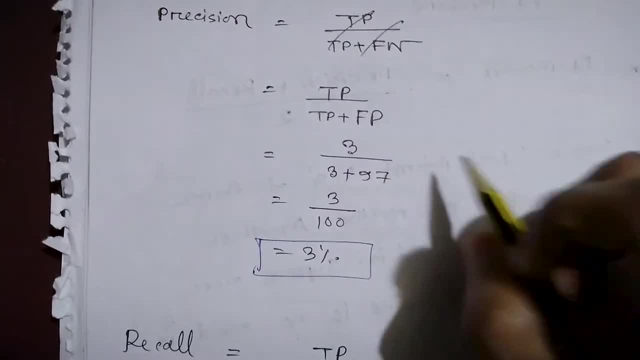 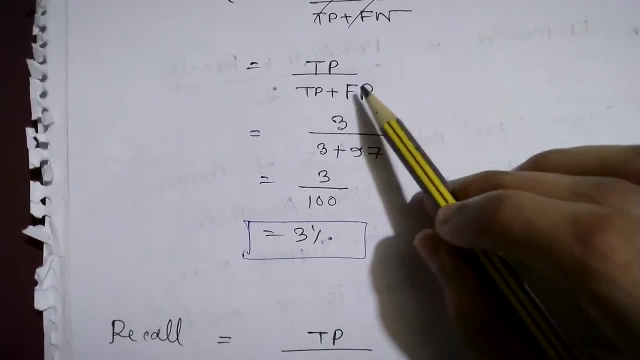 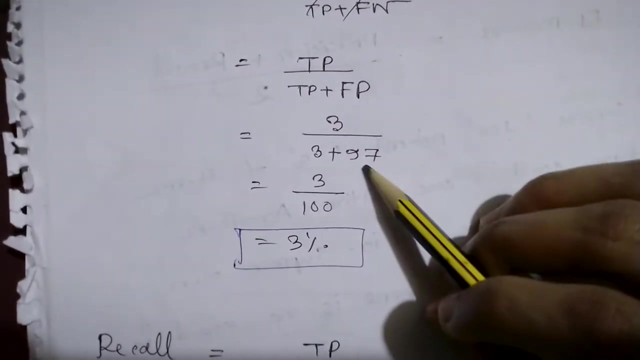 measure. so to the first normal for precision is tp divided by tp plus fp, which is true positive divided by true positive plus false positive, true positive is three. so it actually says that when false positive is actually the negative value, false positive is actually a negative thing. it says, actually you do not have 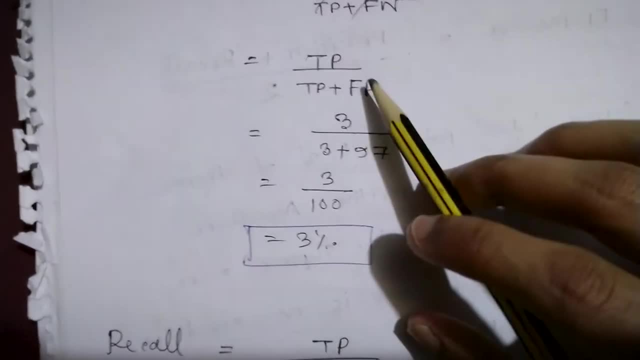 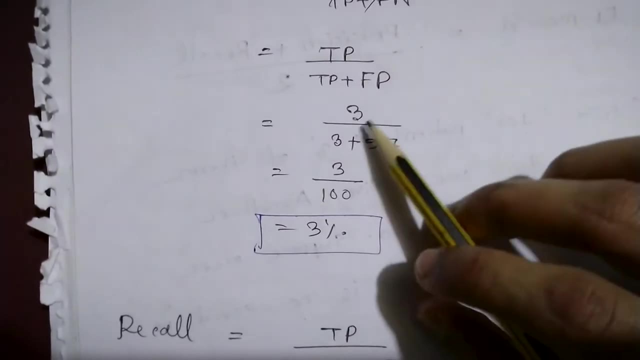 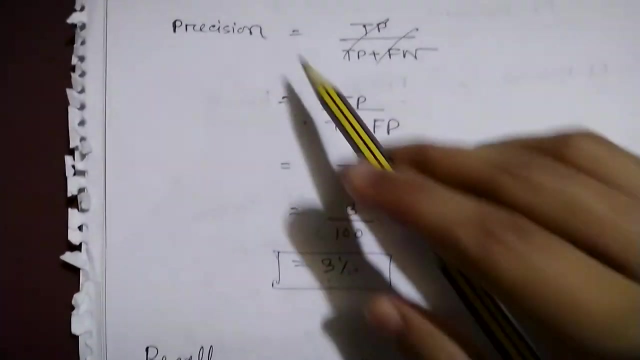 97 of them do not have governor virus actually. but your model predicted that 90, 97 of them actually have gone over your model predicted. but actually 97 is the part that you do not have gone here. so false positive is 97. so 3 divided by 100 is only 3 percent, so your precision is on. 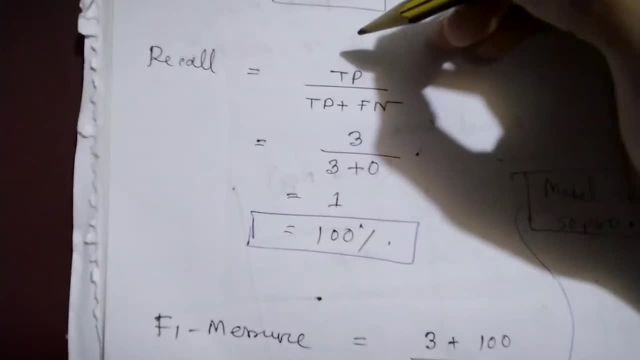 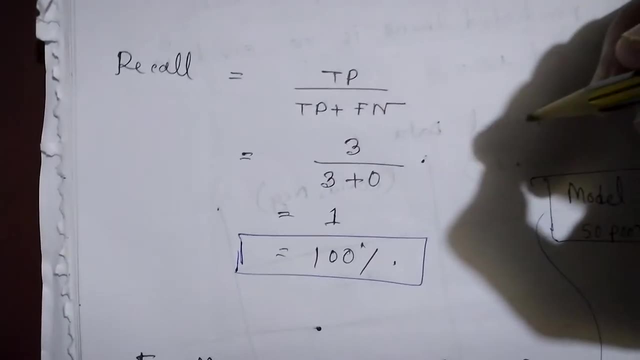 the only 3 percent very low. let's find the recall. recall is TP divided by TP plus FN. this is true positive: 3. true positive is 3. false negative is 0. why false negative is 0? let's see, so this is your false negative, when actually you. 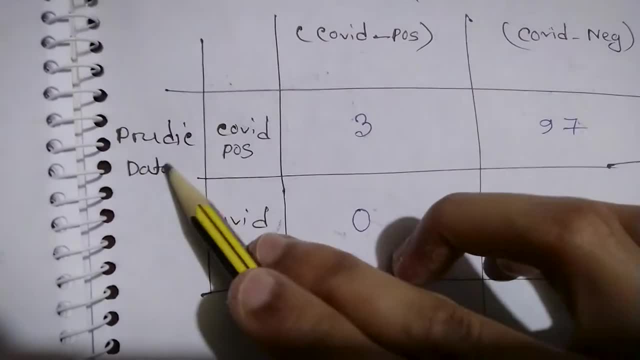 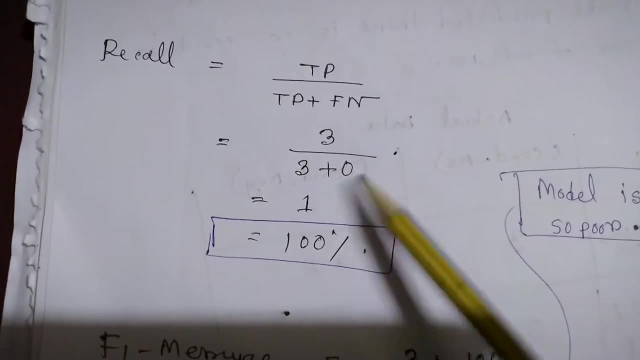 have positive, but your copy 19 model predictions is 0, so this is false negative. so we're false. negative is 0, so 3 divided by 3 plus 0, which is 1, which is 100 percent. you recall is 100 percent. so let's find F1 measure. F1 measure is: 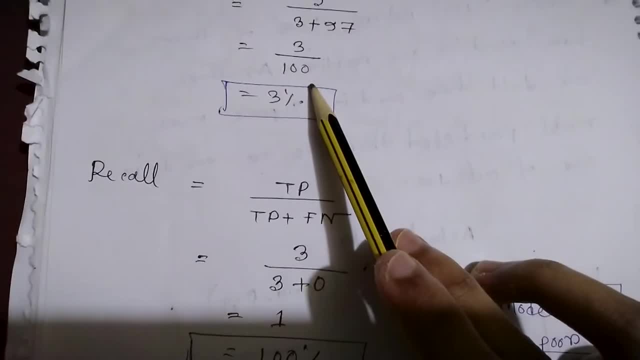 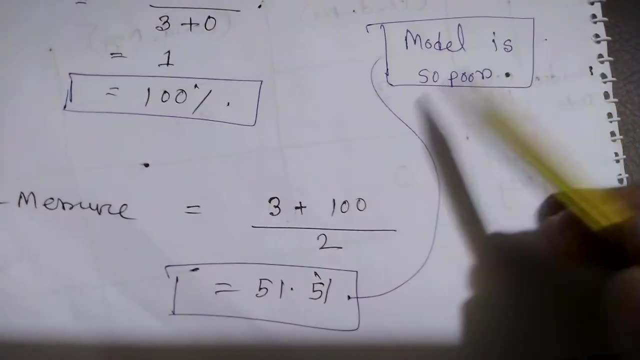 the precision plus recall, which is 3. this 3 precision plus this 100 recall, 100 divided by 2, which is 51.5 percent. so your model is not that good. it is very poor. it is only giving 50 percent of the chance. there is another technique. 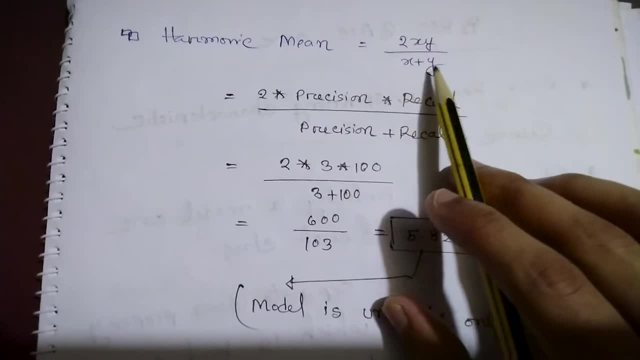 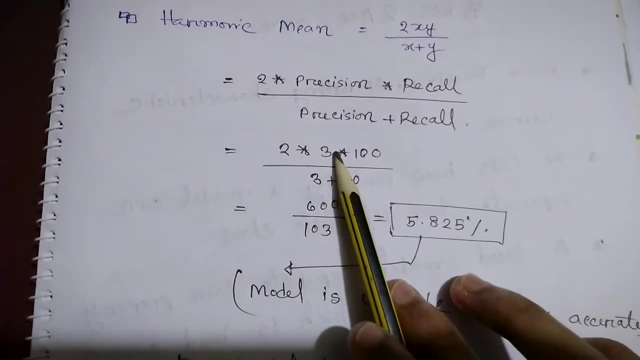 which is harmonic mean. its formula is 2 X Y divided by X plus Y, so 2 times precision times recall, divided by precision plus recall. this formula is really simple: 2 times precision is 3 recall is 100 divided by 3 plus 100, which. 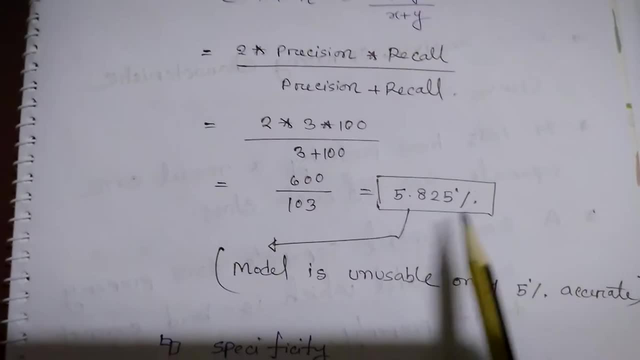 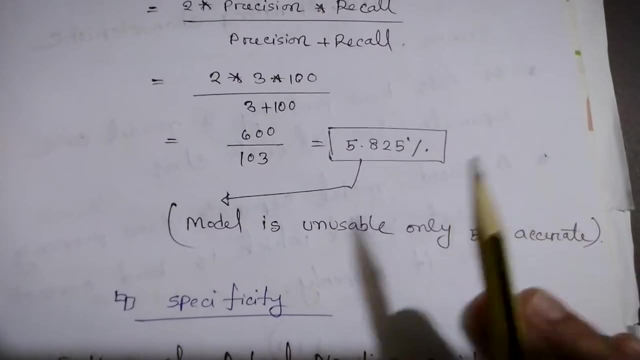 is their sum, you get 5.8 to 5%. this harmonic mean is say that this model is unusable on the 5% accuracy. it is only 5% accuracy, so we cannot use this model. to use this model we need to use 96, 97, 98 percent accuracy, but it gives only 5. 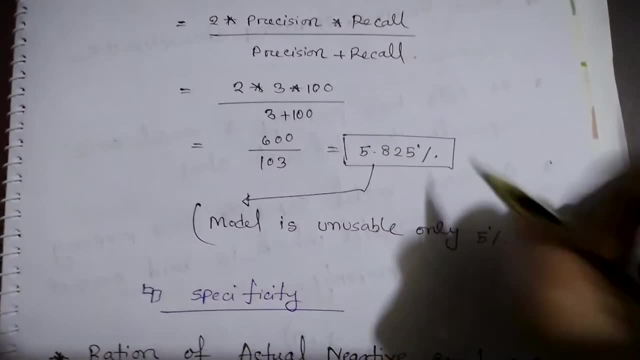 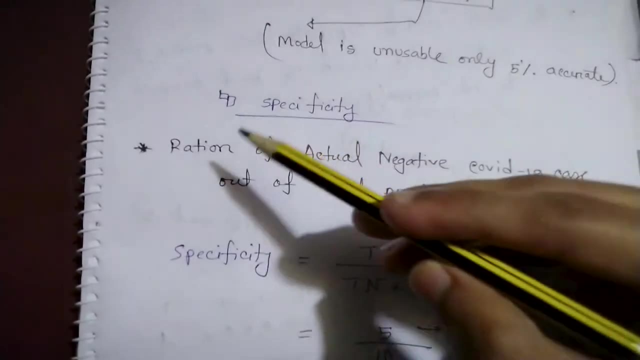 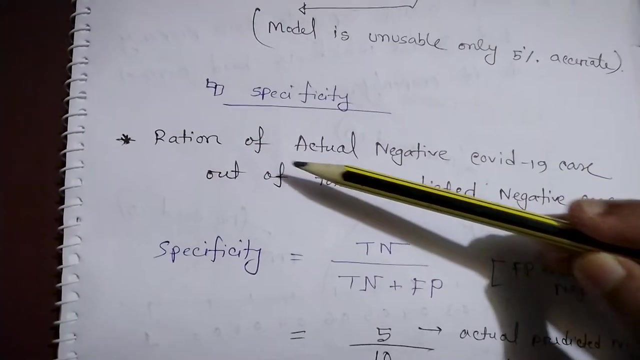 percent accurate. so it punishes the model that it is only percent accuracy. we cannot use it at all. it is unusable. so let's, so let's get. so let's understand the specificity. specificity works with the negative values, but recall and precision works with the positive value. so it specifically means that the ratio, the actual negative covenanting, 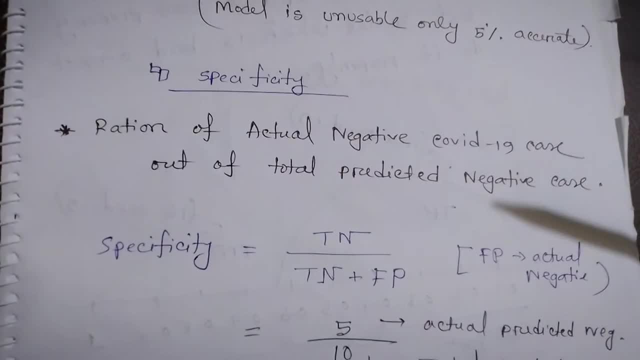 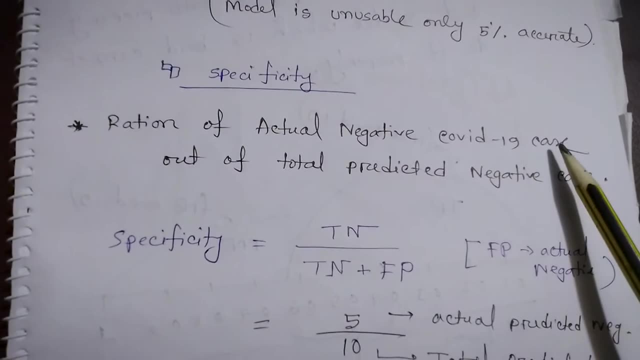 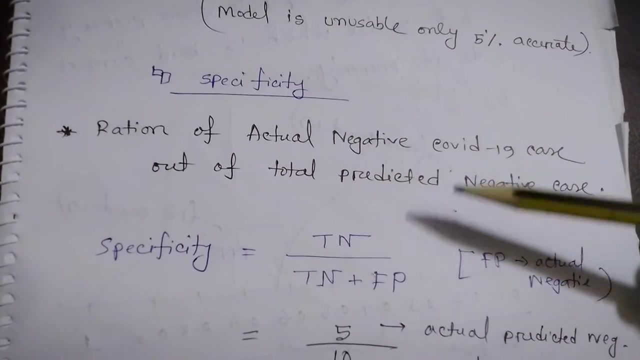 case. suppose actually we have five patients which is covered negative. but out of that total predicted negative case is 95. suppose so the ratio of the actual negative covenanting case out of total predicted negative case, total negative negative case is the total predicted by algorithm. it is not actual value, it is predicted by algorithm and in the upper side, 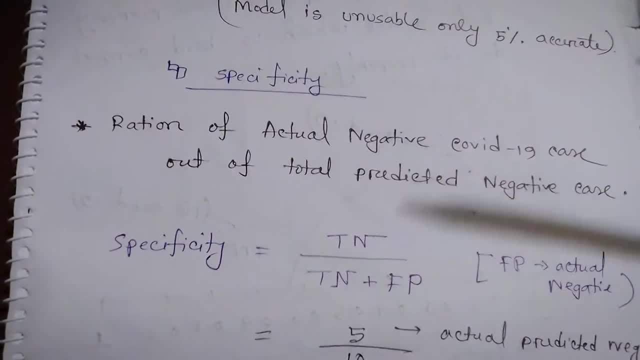 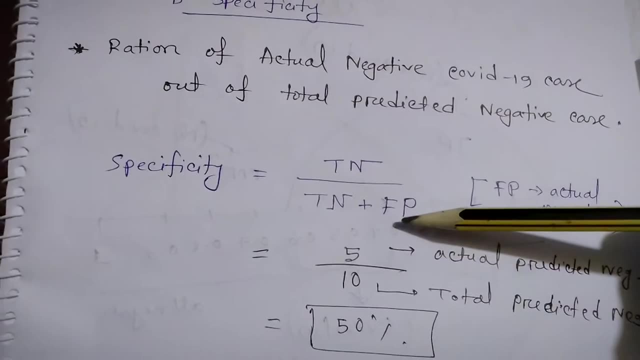 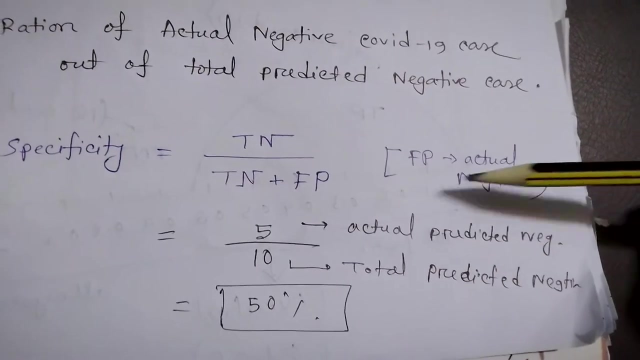 we will have actual negative covenanting case. it's real time, okay. so specificity works with the negative values. so we have true negative divided by true negative plus false positive. so what is false positive? actually it is a negative thing. false positive. your algorithm predicted negative, but actually it is positive. so we need the false positive. 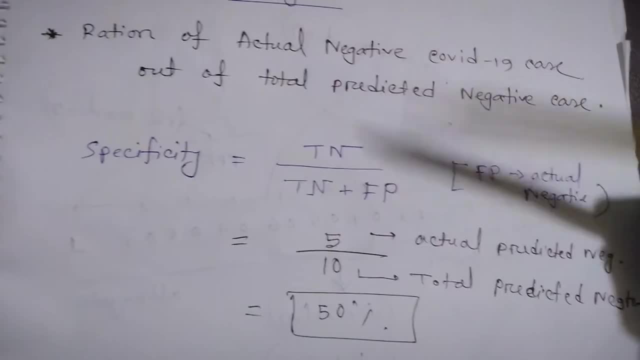 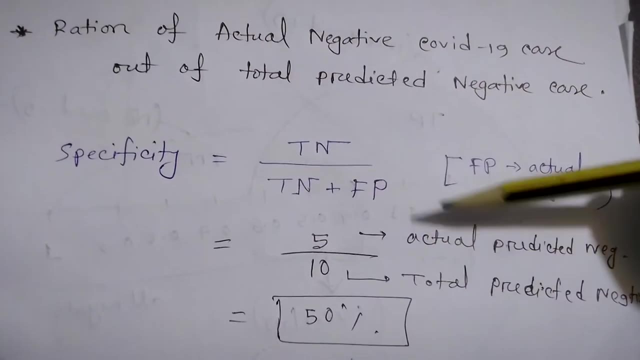 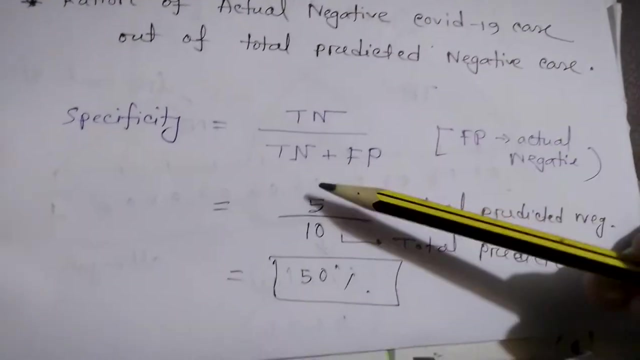 false positive is actually the negative. okay, so remember that false positive is actually the negative thing, but your model predicted as it is positive, but actually it is a negative thing. it says actual negative, but your model predicted positive, so remember that. so true negative suppose five. okay, divided by true, negative is actually the five, because 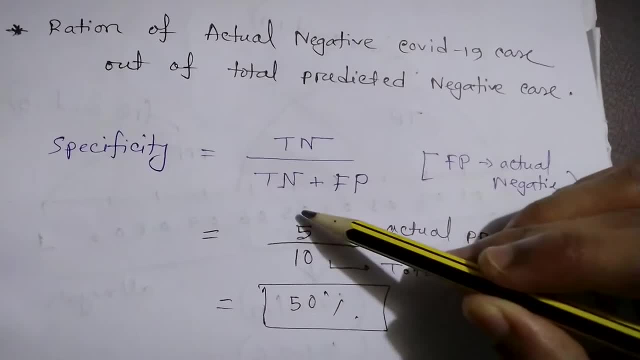 five is actually the negative. so true negative is actually the positive. so true negative is true negative is actually the positive. because true negative is actually the positive. so true negative is actually the positive. so true negative is actually the positive. so true negative of them actually have covenanting. plus false positive, total negative. actual negative is 5. 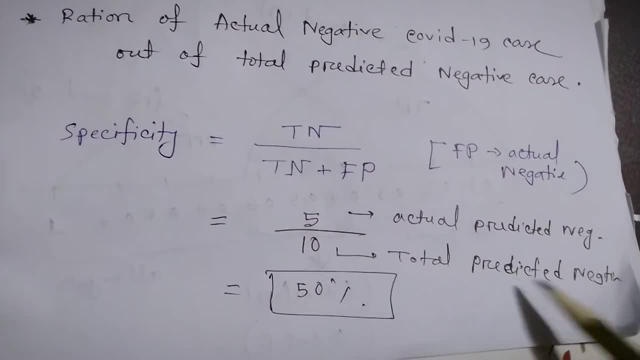 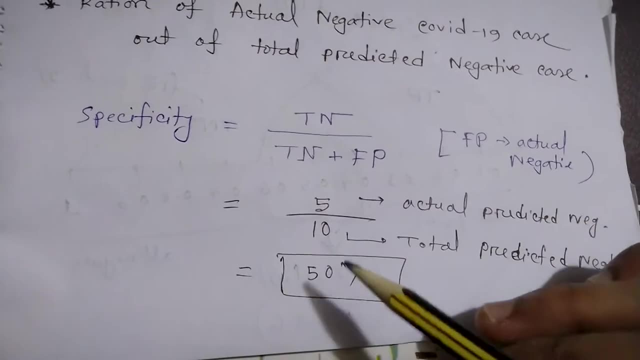 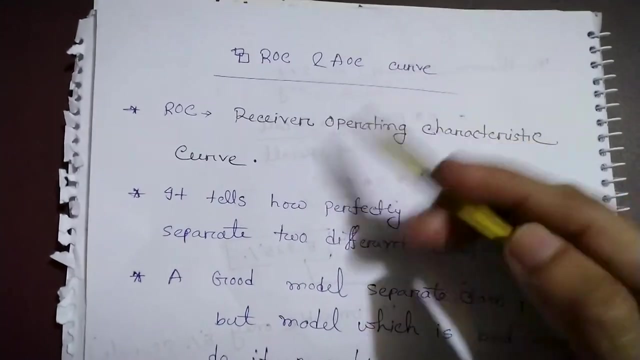 true negative out of the total negative. suppose total predicted negative is 10. okay, tn plus fp is 10, so we get 50 specificity. okay, this is the accuracy of 50 percent for the specificity. so, guys, this is really important. rock curve and eoc curve: okay, so rock curve is actually. 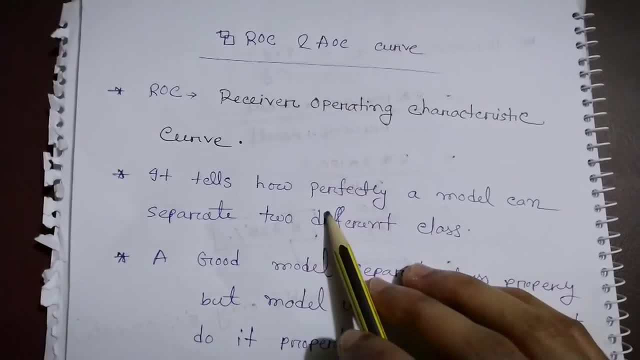 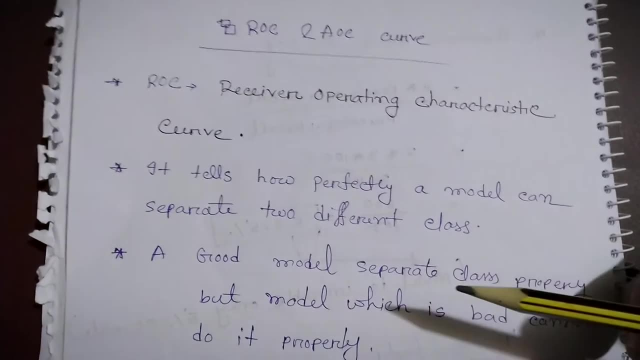 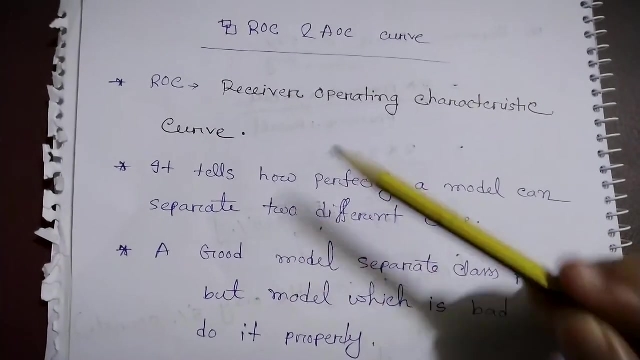 the receiver operating characteristics curve. it tells how perfectly a model can separate to different classes. we need to classify those two different classes based on different kind of performance metrics. how smoothly we can do that, how smoothly we can classify those two different data sets, how we can classify those two different class easily. it tells that. it shows how we can. 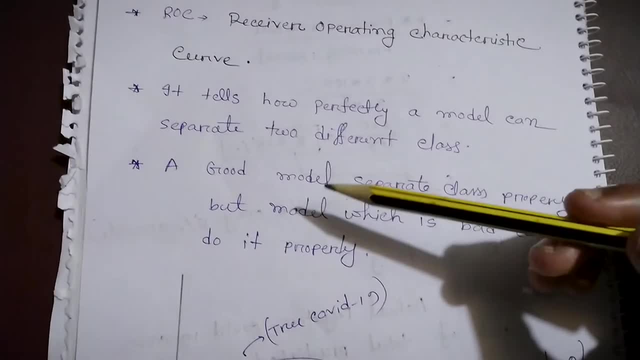 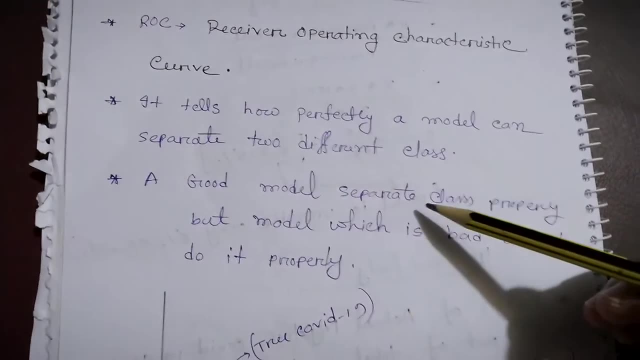 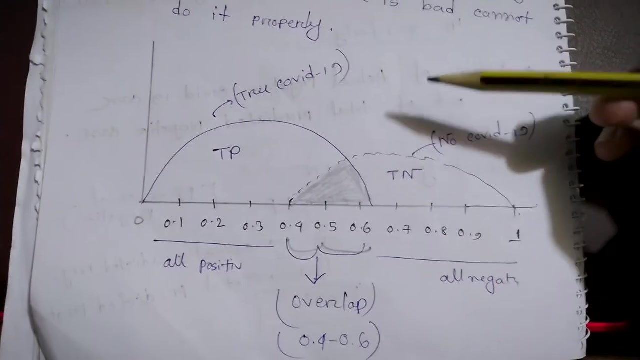 do this effectively. so with the knowledge of precision, recall and confusion, matrix and many other things, we can really understand it perfectly. so a good model separate class properly, but a model which is bad cannot do it properly. so let's understand this diagram where 0 to 0.6, we have the true. 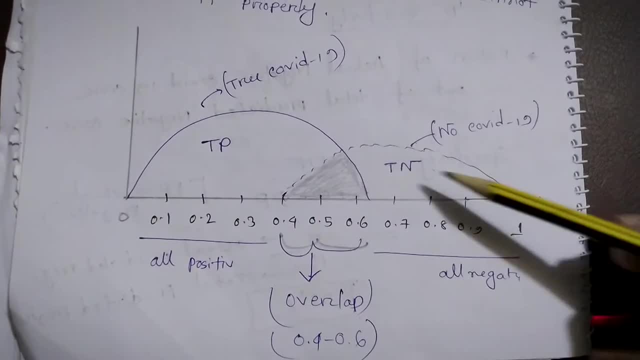 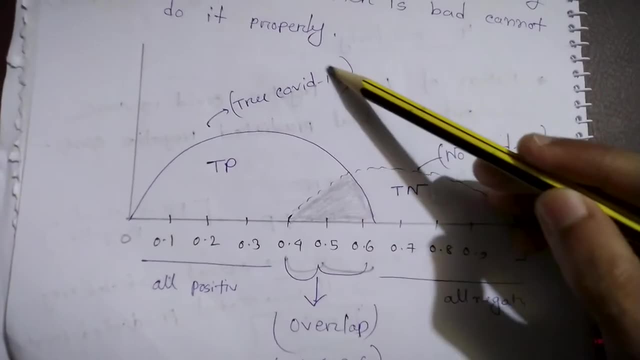 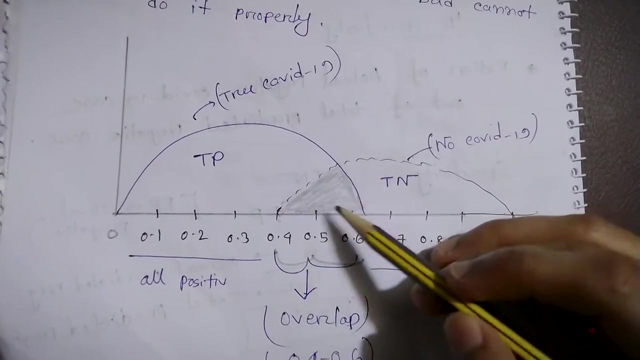 positive value and from 0.4 to 1 we have true negative value. there is no covid-19 in this region and in this region we have true covid-19 case. but look at this: this is the problem. this overlap position is our fault, okay, our model's fault. 0.4 to 0.6, our model fall down. 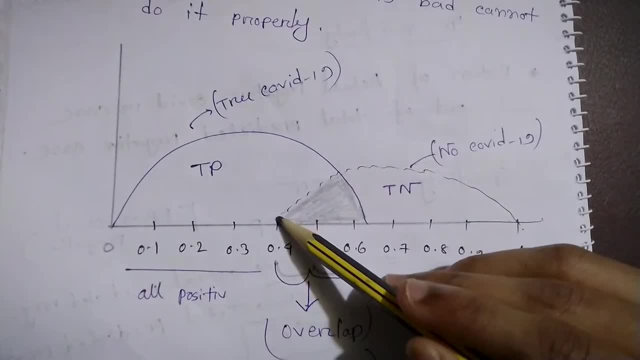 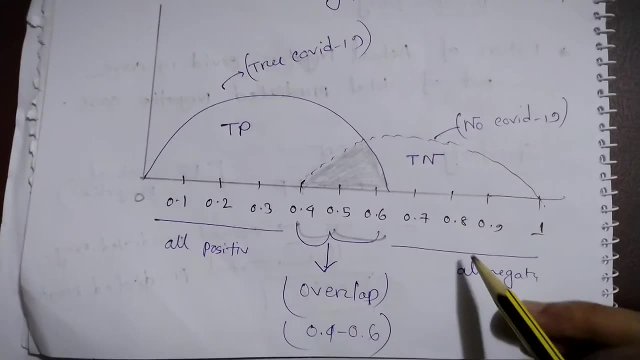 so this is not good for our model because this person is overlapping with true negative and true positive. so this is the problem. so in the left side we have all positive, in the right side we have all negative, but in this middle portion, where we have overlap this position, this range, we 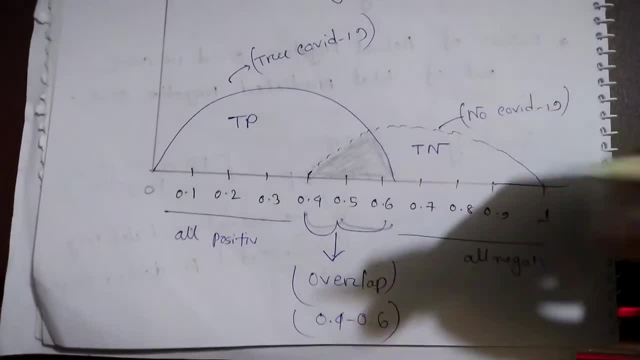 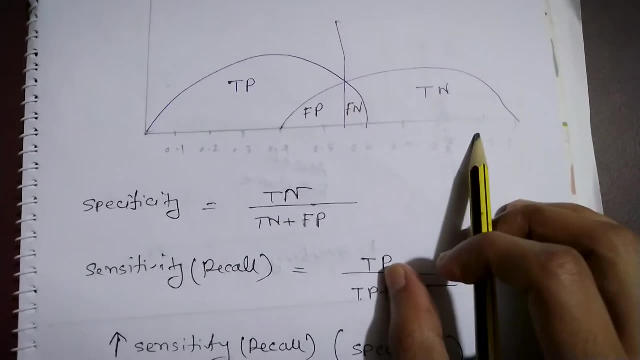 have overlapping. so this is the problem that we need to remove. we have different kind of case. in the left side we have all the true positive up to 0.6, and from 0.4 to 1 we have true negative. but when we do a classification here, within the true positive we also have the false positive. 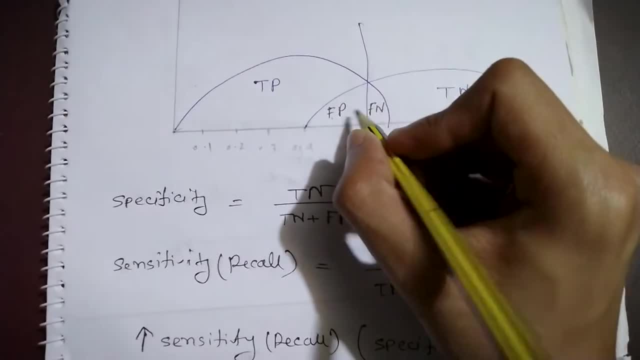 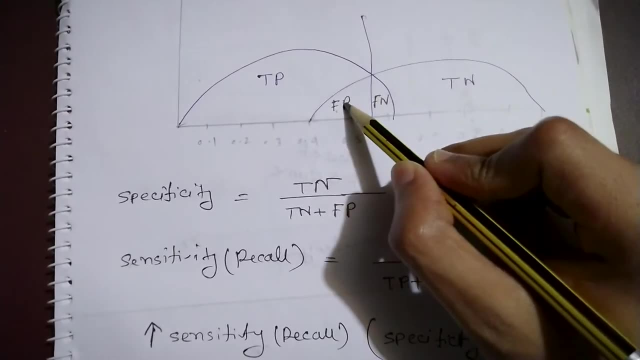 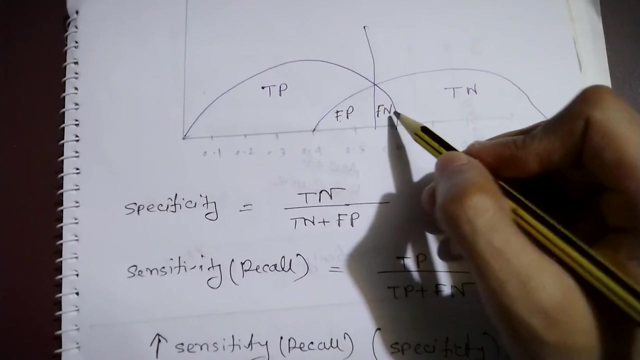 false positive is actually a negative value, so that we do not have. actually this is under the true negative, so it is a negative portion we. this is the problem and for true negative, the problem with the false negative: false negative is actually a positive value, actually positive, but you. 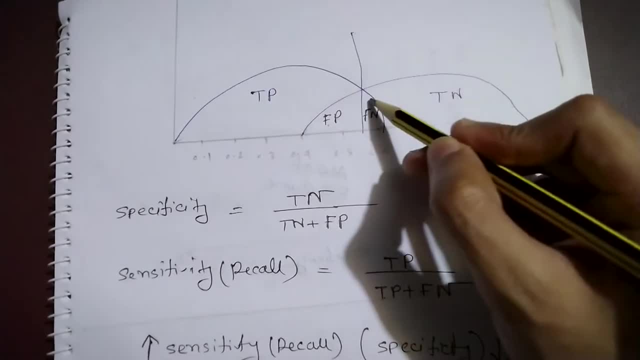 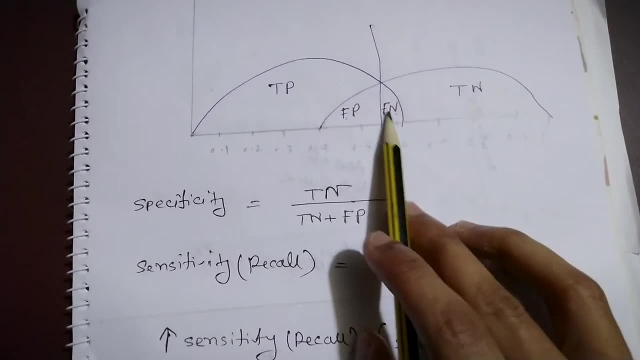 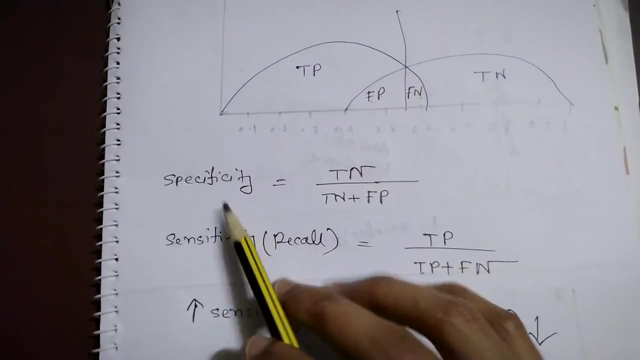 model predicted false. okay, so this is the problem we have. so with the true negative, the problem is false positive, and with the true positive, the problem is the false negative. so we need to remove those kind of things. so this is the problem, okay, so it specifically works with. 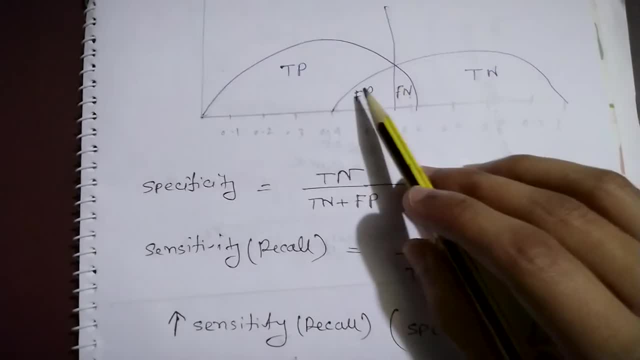 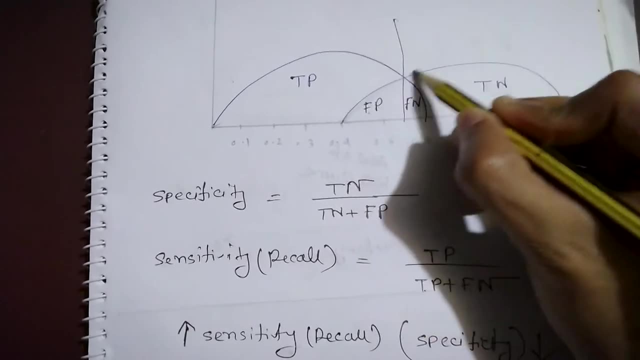 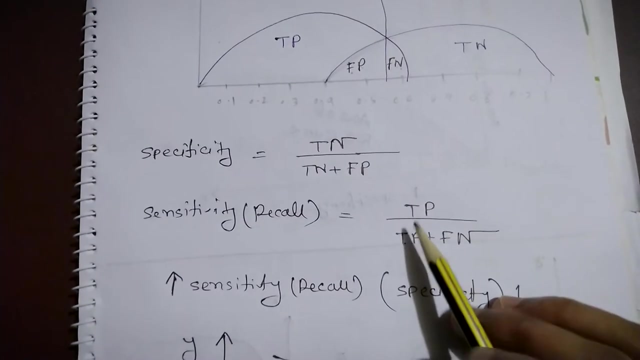 the negative value, true negative everywhere. true negative plus false positive. so this two curve- false positive- is actually negative. so this portion is actually the portion for negative, not true positive. okay, so we need to add that. so true negative divided by: and its sensitivity is actually- we can also call it as recall- works with the positive value, so true. 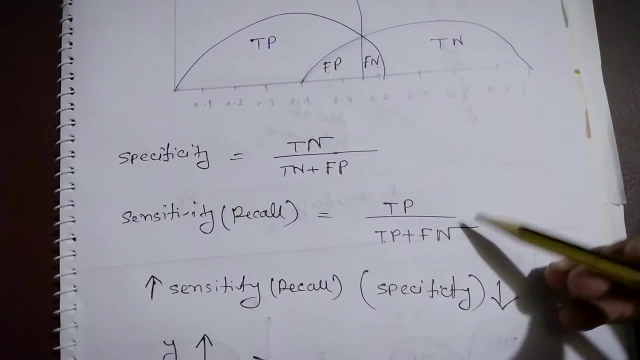 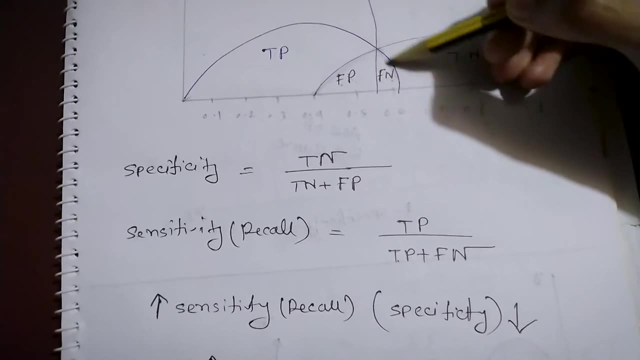 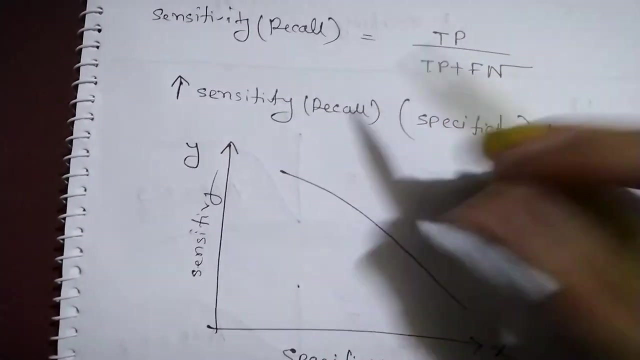 positive, so true positive divided by true positive plus false negative, so this false negative. okay, so this portion plus true positive, because this portion is a portion of true positive, not true negative. okay, so this is the thing that you need to understand. we can call it sensitivity as recall. 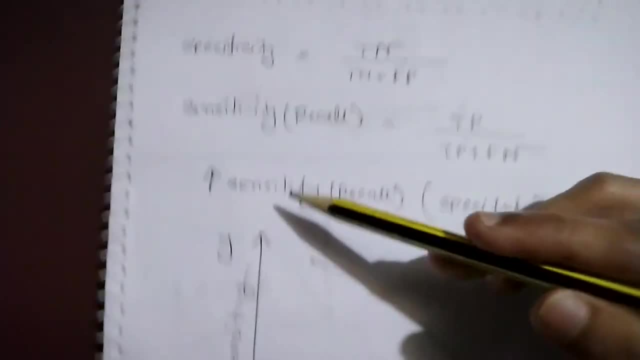 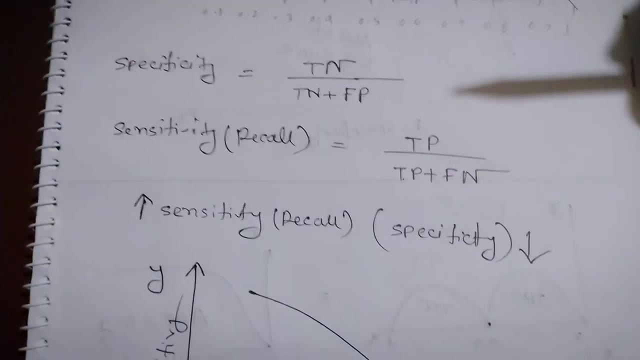 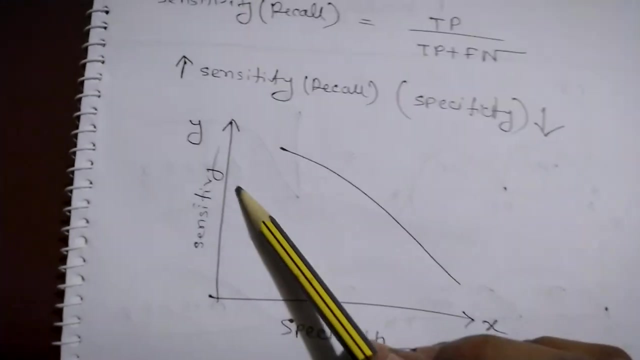 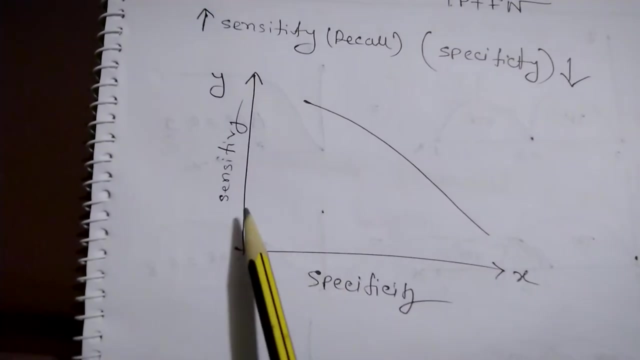 as well, and we can call, we can understand that specificity works with true negative sensitivity, or recall works with the true, positive. okay, so we need to draw a curve here. specificity is actually specificity and sensitivity- this is actually the recall- when, when we get, the specificity is higher. as you can see here, the sensitivity is lower when the specificity is. 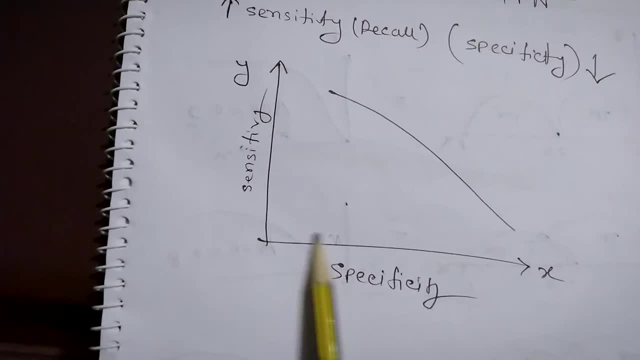 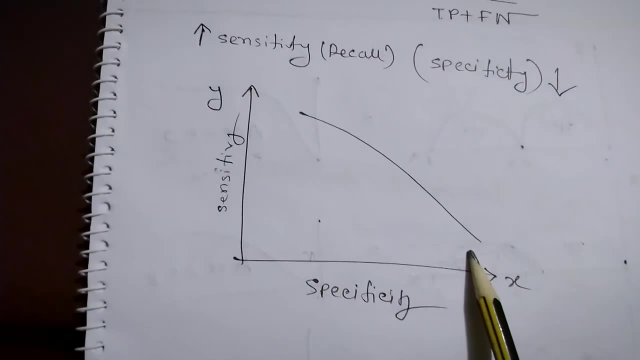 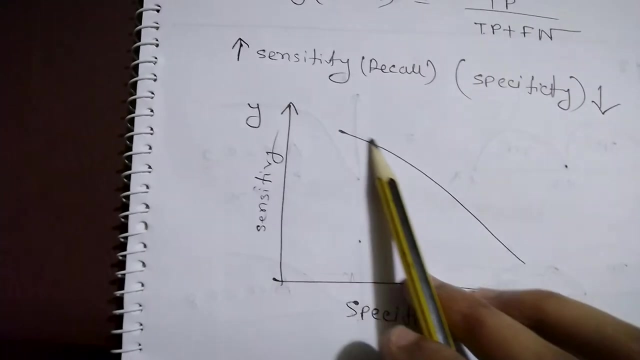 lower, the sensitivity is higher. so we can say, when we increase the specificity, specificity is actually when we work with true negative and the true negative increases the sensitivity, the recall decreases. this recall decreases. as you can see, the recall is decreasing with the increasing in specificity, with the negative value increasing. okay, when you increase this value, this value, 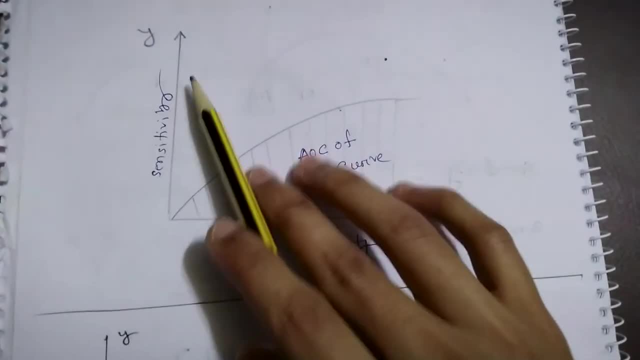 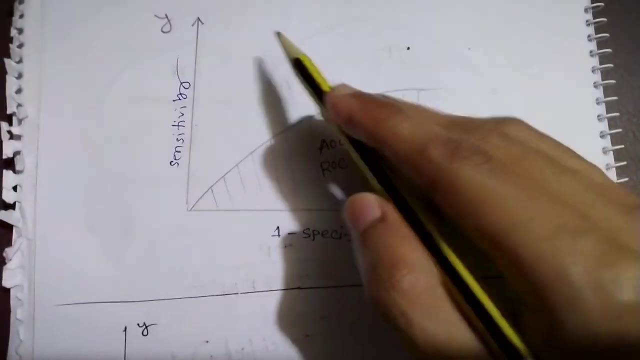 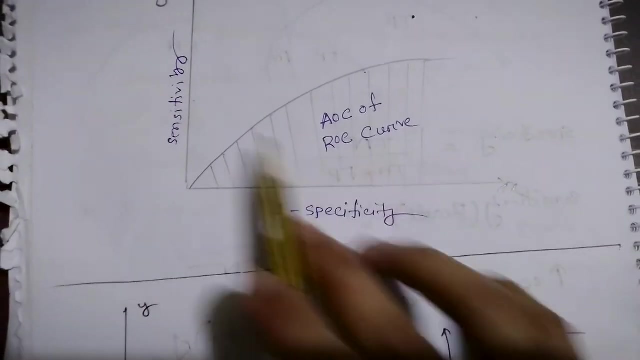 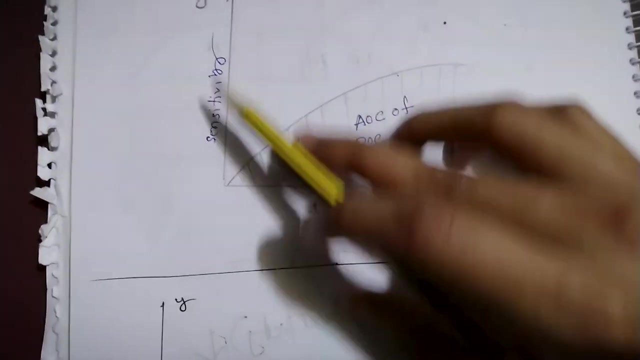 decreases. so there is inverse relationship. so from that relationship we can get the aoc density curve, aoc of rock curve. so sensitivity versus specificity is inverse relationship. but when we draw a graph with one minus specificity it means that this value and this value are the linear way. it is positively curved. when this one minus specificity increases the sensitivity. 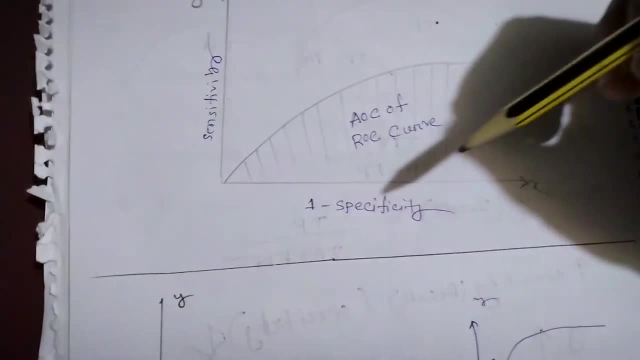 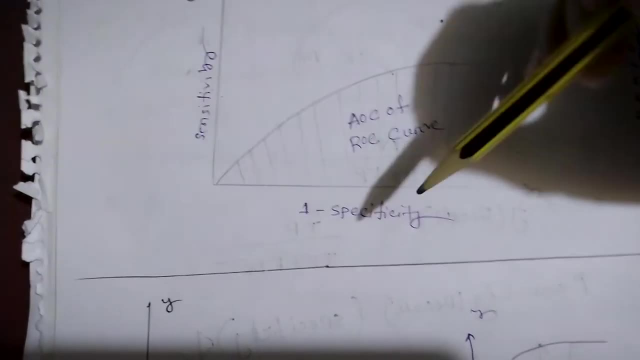 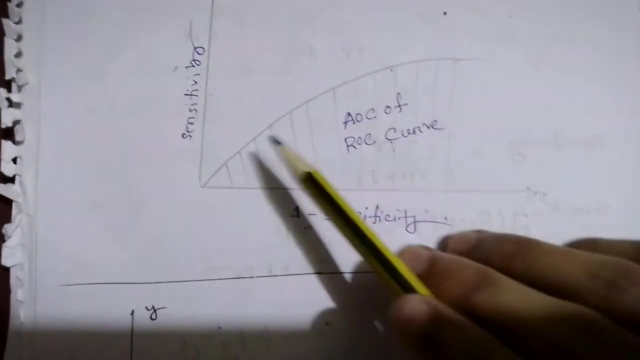 increases because specificity and sensitivity are opposite. but when you do one minus specificity, it means that it is also positive increasing. and this is also positive increasing because we know that specificity, specificity, works with the negative value. but when we say one minus specificity, it becomes positive. so our graph becomes this way. from this way, our graph becomes this way. 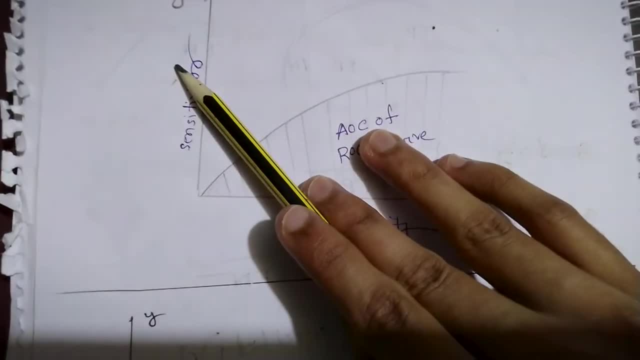 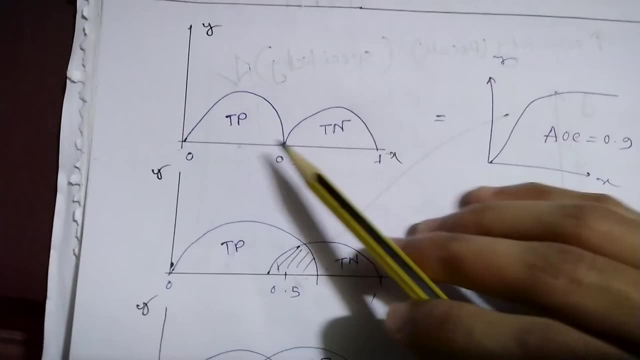 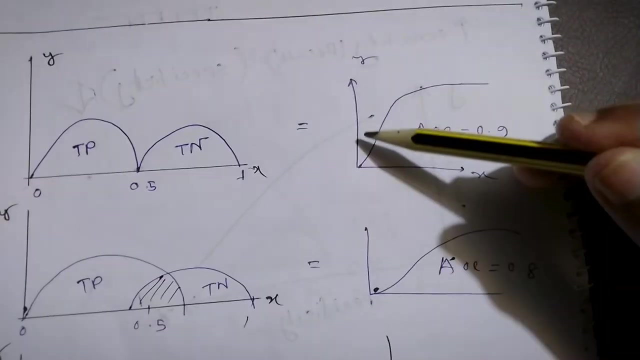 when the specific one minus specificity increasing, sensitivity also increasing. so they're definitely positively correlated. okay, so see that these three graphs, when zero to 0.5, we have true positive and we have true negative to 0.5 you. so there is no overlapping. so our aoc curve gives this way straight curve which says zero. 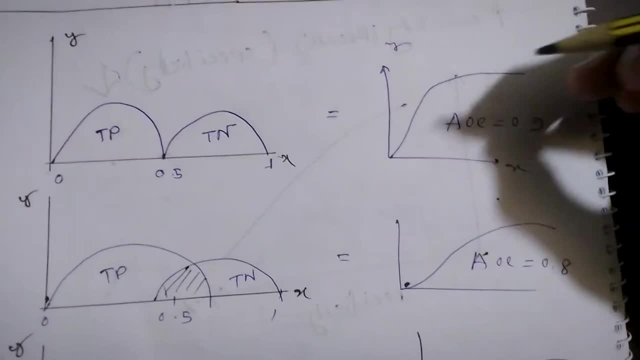 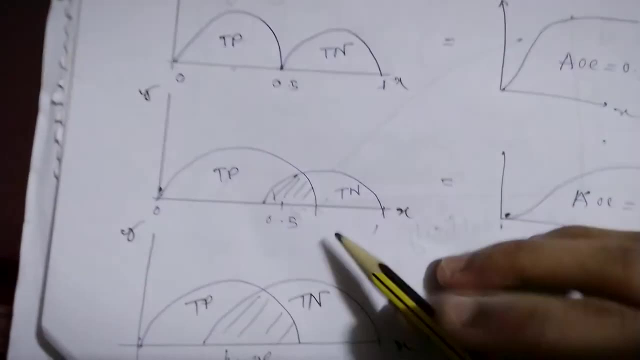 aoc is actually 0.9, which means- which means that is a very good model. we can separate those two classes with a straight line property. okay, there is no overlapping here, but here we have some overlapping. we have false positive and true negative here mixed up. okay, so in this case, 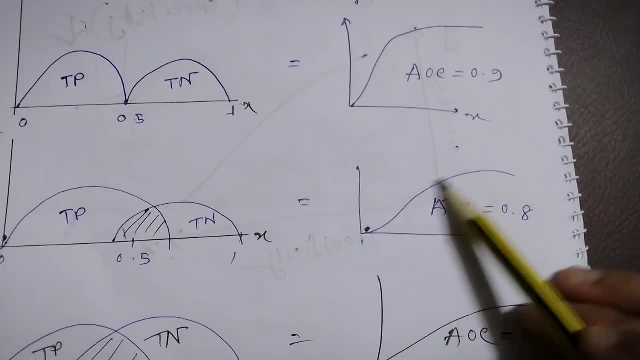 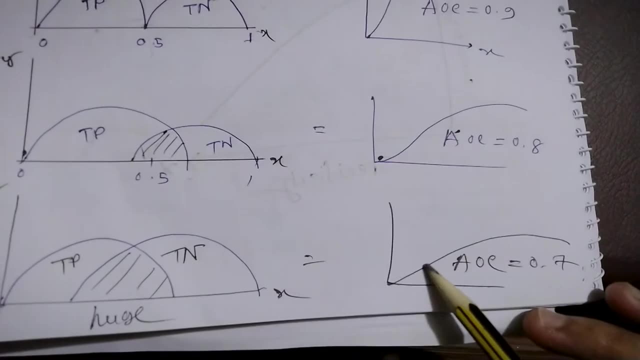 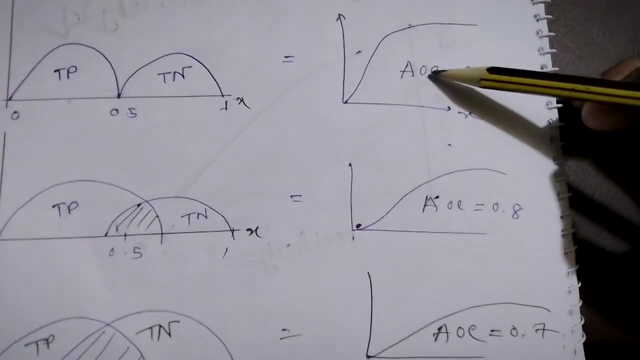 our aoc is slightly in narrow down here to the x-axis. it says aoc is 0.9 when there is a huge amount of overlapping. it also narrowed down near the x-axis, which is 0.7- 0.. as you can understand that when the eoc is higher, your performance model is very good and 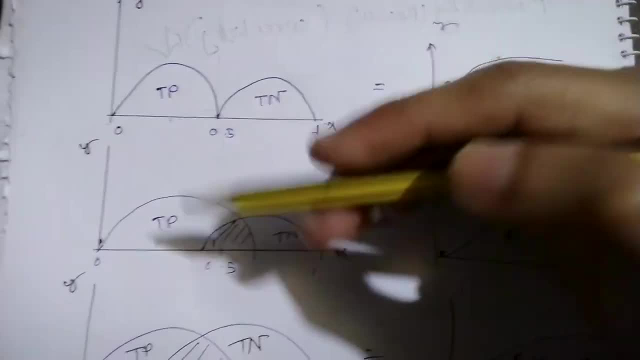 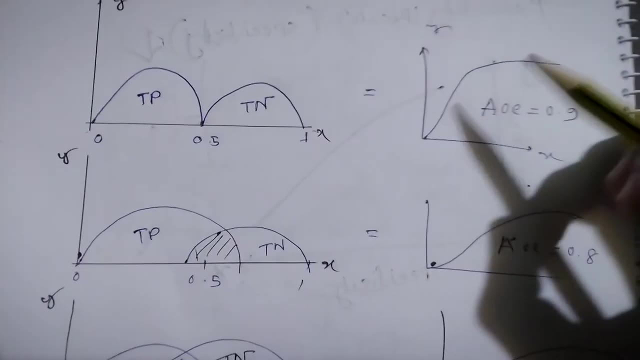 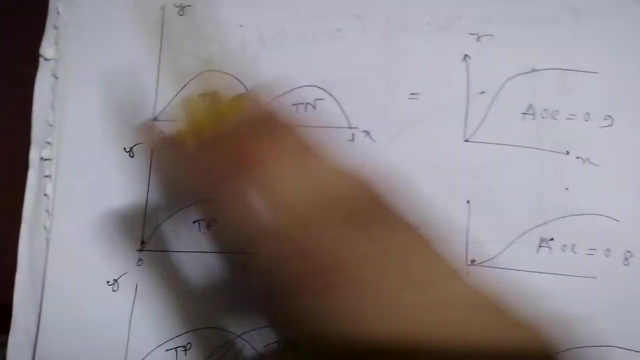 you get better accuracy because it can differentiate your model with the true positive and true negative equal number of times and it is better to classify two different classes with this model, which is what our primary model, our primary intention, should be: two different to different, to classify to different classes with a single line, with a single line drop here, but here we cannot. 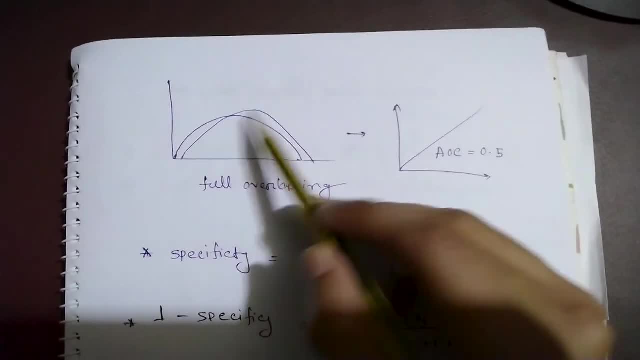 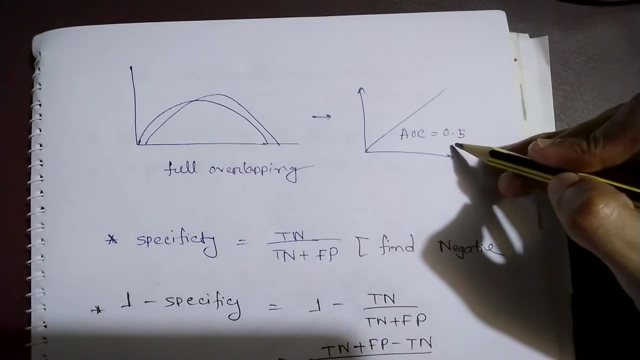 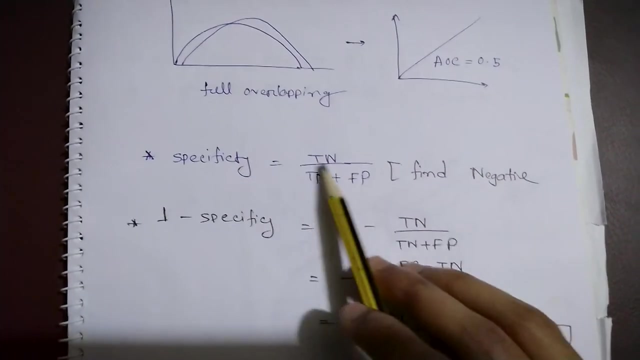 do that overlapping. so in this case, true positive and true negative are completely overlapping each other. in this case, that what eos ud is straight curve, okay, straight line. so it says 0.5 whenever eos is 0.51. model is very bad, it is trash, it is unusable. so, as you can see, specificity is to work. 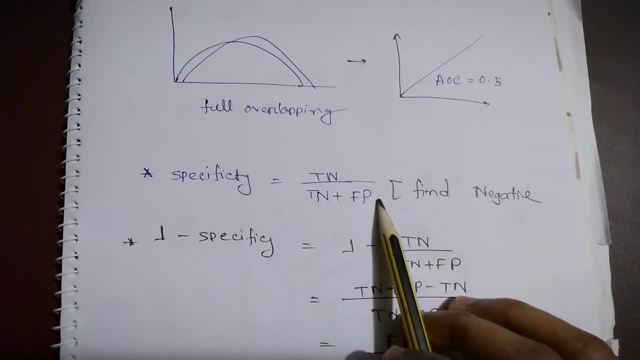 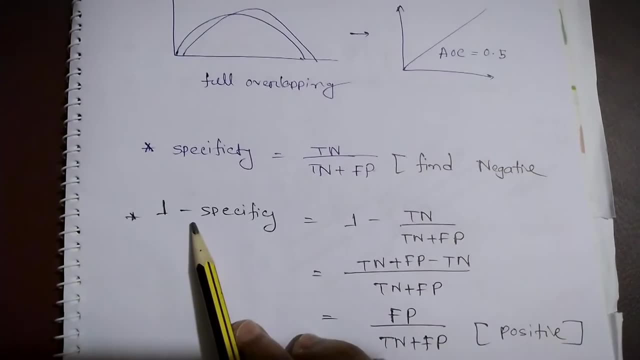 with negative, true negative to negative plus false positive. false positive is also a kind of negative, actually negative value. okay, so we are working with the total negative. so when we say, when we say one minus specificity, which is one minus this value, then we get. when we get the calculation, we